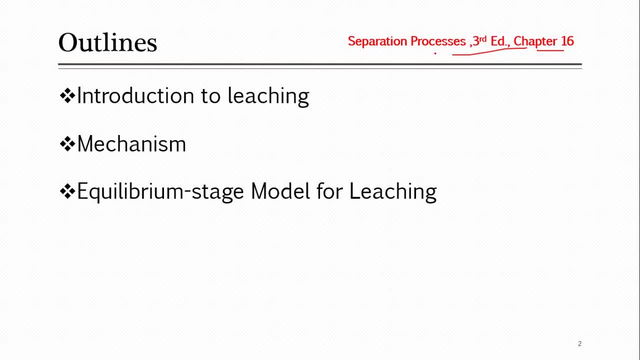 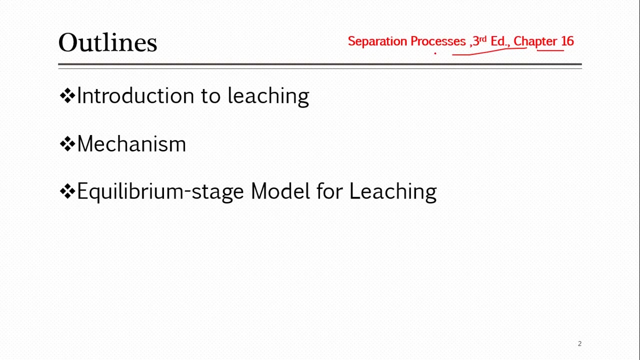 Membranes, then there were gas separation membranes and finally, in the last lecture, we discussed pervaporation membranes. Before that we discussed liquid-liquid extraction and before liquid-liquid extraction, actually absorption was detailed and discussed throughout the seven weeks or eight weeks before midterm. 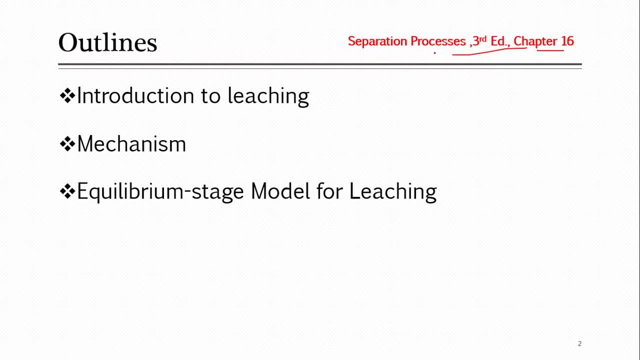 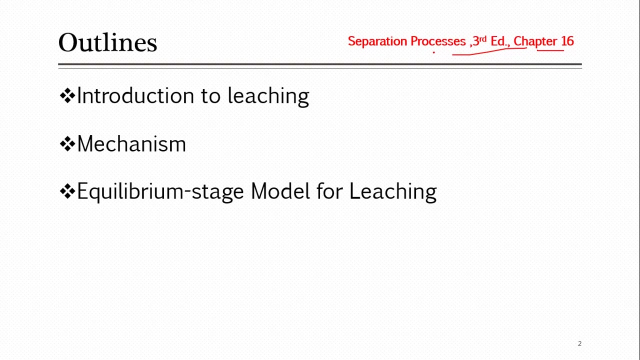 So this last topic which we have to cover overall- Here I am just going to cover major introduction and this equilibrium stage model, or they also called it sometime counter current washing model. So this we are going to cover, but only one thing which will be left. that was related to mass transfer phenomena in the leaching and the numerical stuff related to that which we can't cover, because this is the last lecture in which I will just introduce you with the leaching. 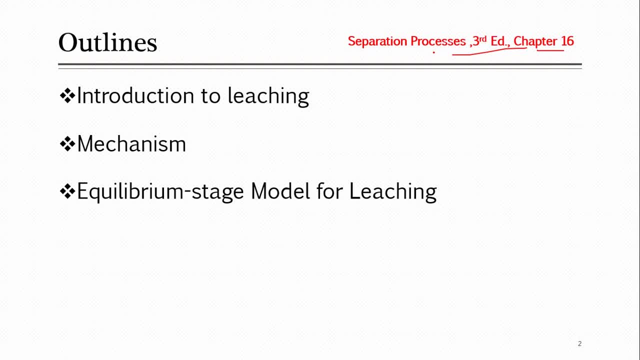 And we can't cover that only one topic. So overall, Alhamdulillah, we have done well throughout this pandemic and everything. Alhamdulillah, we may need to cover our syllabus, So let's start with this leaching. 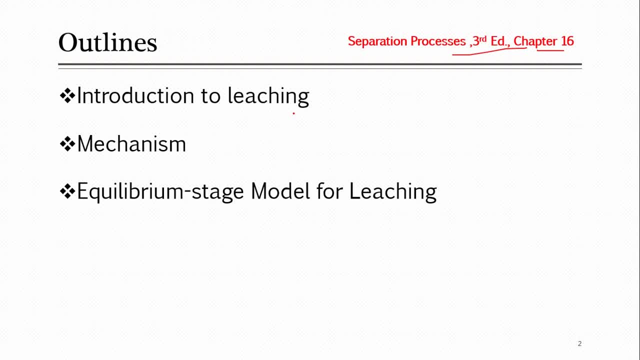 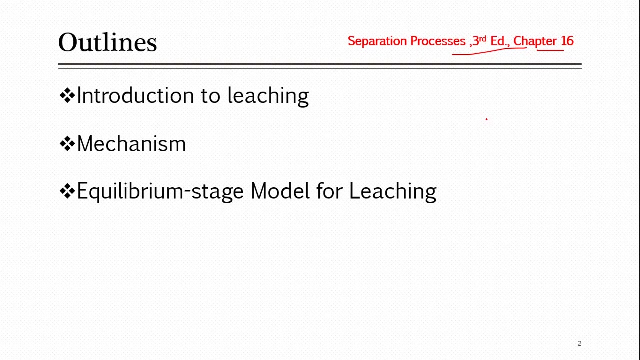 What is leaching or what is this solid liquid extraction? Before this you studied liquid-liquid extraction. So just to recall, liquid-liquid extraction actually involved two liquids. One liquid was Our feed and if you remember at that time, the liquid which was feed, that consist of two parts: one was carrier and other was means, some solute inside that feed and an external liquid. another liquid was introduced to the system and that was named as a solvent. 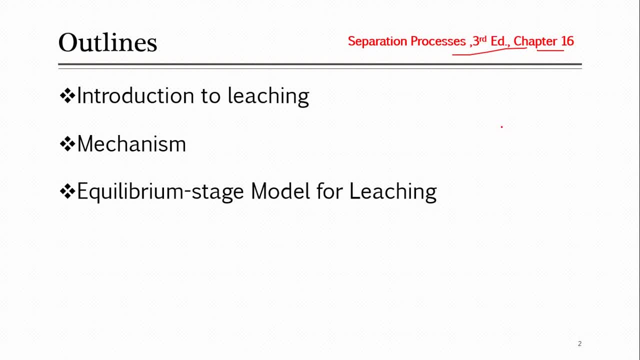 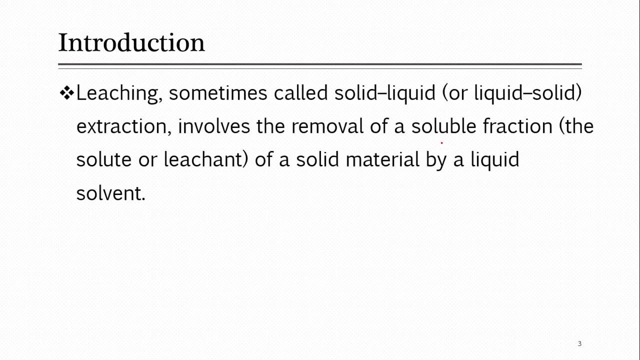 So that solvent actually extracted some components from this feed and those component were extracted which we were looking to be separated. So here, somehow same thing which we are going to have, that's the solid-liquid extraction. so inside this, let's look. what does this mean? leaching or sometime also referred as solid-liquid or liquid-solid mean- any name you can give it. extraction process involved the removal of soluble fraction of a solid material by a liquid solvent. 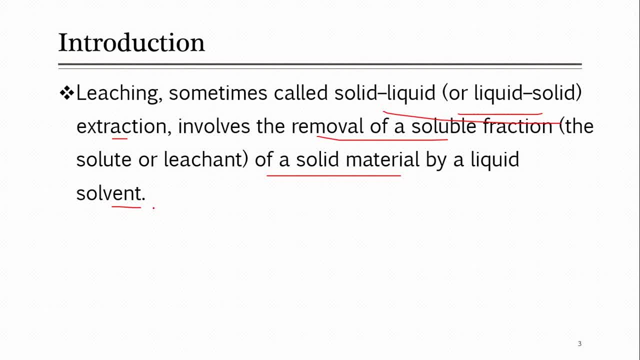 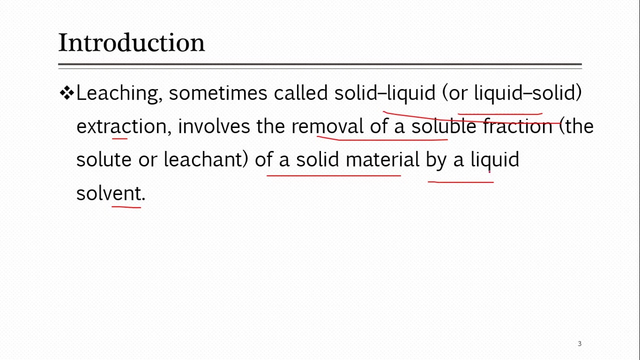 So it is somehow similar to the liquid-liquid extraction that in the liquid-liquid extraction you used to introduce some external solvent Or a liquid. so same here: you are introducing external solvent or a liquid and you are extracting, you are removing some part of the solid material or mean- removal of soluble fraction of solid material with the help of this liquid mean. if I compare it with the liquid-liquid extraction, there was one instead of solid that was liquid, which was existing in the form of feed. we used to call it as a feed. 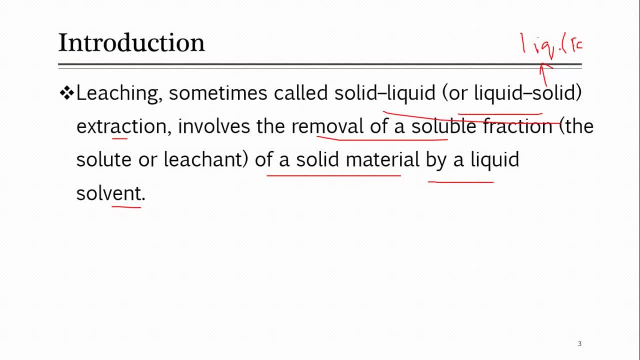 So at that time, that feed consisted Of one some carrier or solvent, as well, as some part was solute, which was recovered or which was extracted by another introduced liquid. so here same, instead of liquid in the liquid-solid extraction, you will have your feed as a solvent. 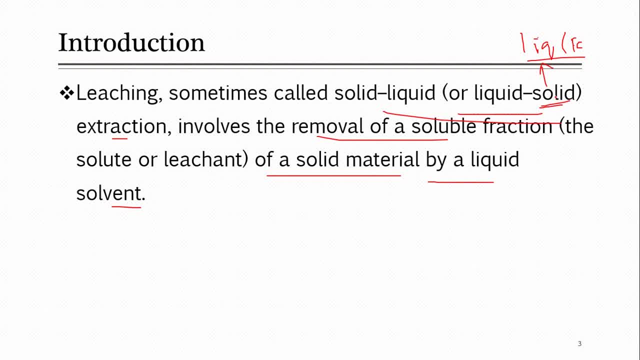 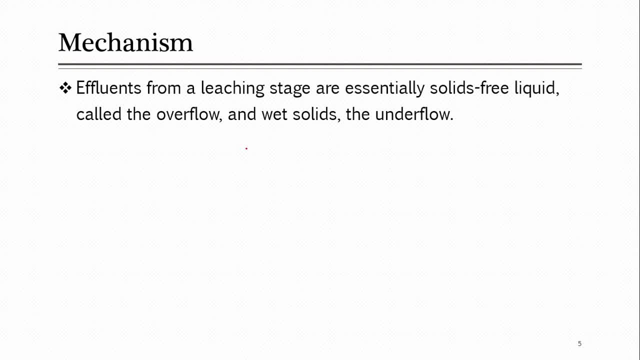 So that feed solid will contain two parts. some part will be like our required part which we want to extract. that's the solid material soluble in this. So at the end, when you have done with the leaching, what you will get that is something solid, free liquid, that liquid which does not contain solid but it contains some part of. 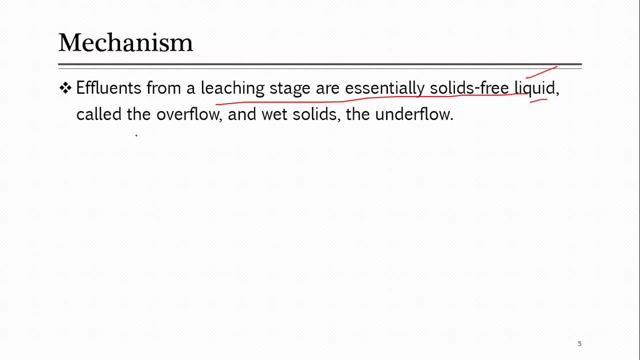 the solid which is now dissolved or soluble inside this liquid. So then this is named as overflow. mean top layer which is separated after extraction, is overflow. that is the liquid which contains some parts of the solid which are soluble but totally there will be, not like solid. due to this we call it like solid free liquid. 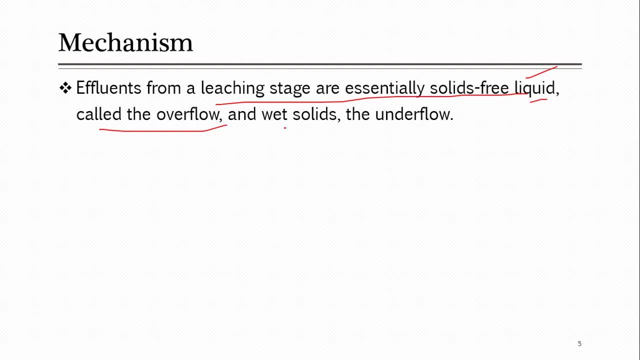 called overflow and there will be wet solids. they leave as an underflow actually the solids which are leaving from that the liquid. sorry, this liquid solid extraction equipment or leaching equipment, those solid usually contain some part of the liquid. due to this he is calling they will be like wet liquid and they flow as a underflow. overflow mean that will. 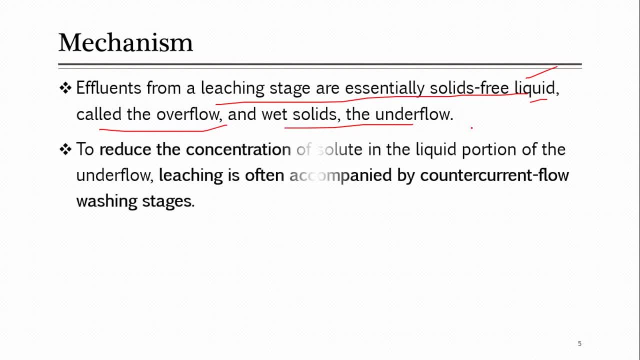 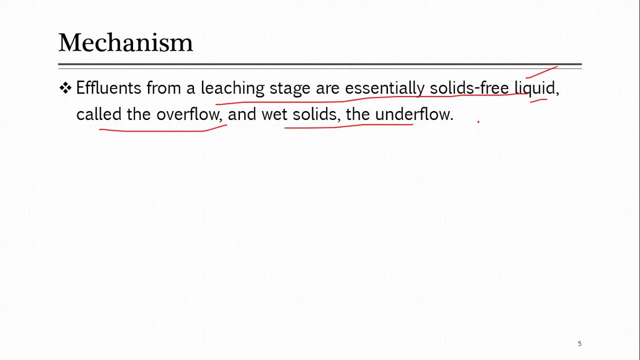 leave from the top of the. So when you extract this in the first stage, for example, you bring in contact these solid with the liquid So that liquid extract some part of those chemical which you want to extract from the solid. So at the end, when solid is leaving from the top, that is, contain some part of those. 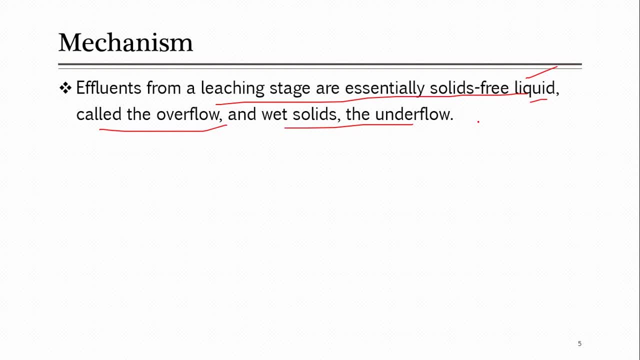 extracted component and it is leaving as overflow but at the same time some liquid it is leaving, as with the solid, as the wet solid. So that will also contain this liquid, will also contain some part of those extracted component, because this is top liquid, is not separate one overall liquid, is homogeneous. 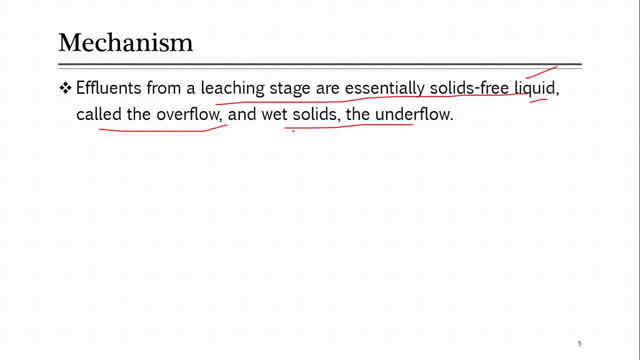 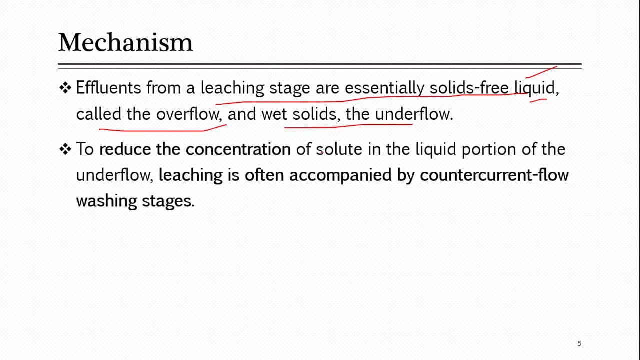 throughout the main equipment. So the liquid which is leaving with the solvents, solids even also contains some part of those solutes, those lichens. So in order to reduce the concentration of those solutes in the liquid portion of the liquid, 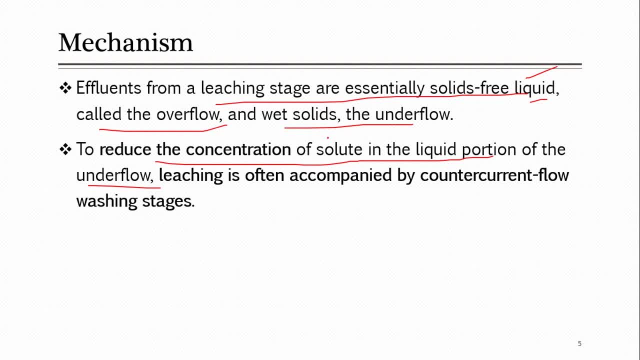 of the underflow. Underflow means this liquid which was leaving with the solid and making it wet So that liquid will contain some part of this solute. So in order to reduce that concentration, leaching is often accompanied by a counter flow washing stages. So sometime this 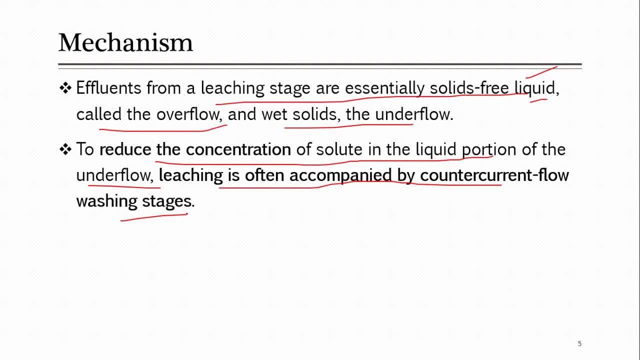 is not only one stage, and most of the time this is not only one stage. you have more than one stages. I will give you the example of this. for example, you dip the tea bag in the hot water. you just mix it up for some time, or give it some time, So that some part of that tea is extracted to your 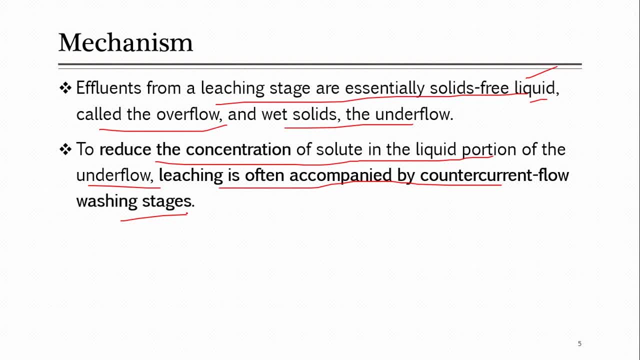 water. Now, after some time, you just take away this tea bag. So when you are taking away this tea bag you most of the time you see you used to sukkies that main tea bag with the help of spoon, So why you sukkies? actually you are just removing the water which was part of this and that water. 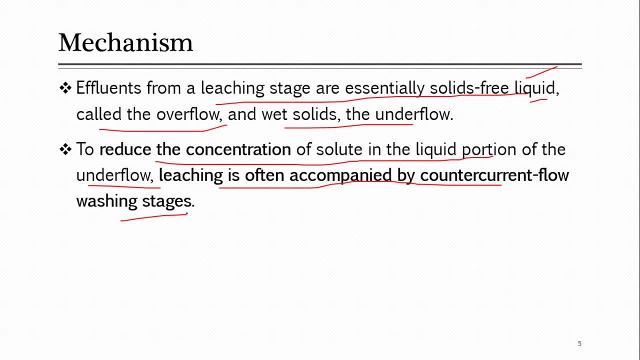 will also contain some parts of this tea which you want to. So that is the, I mean this phenomena of counter current. somehow you can make it like similar, that something counter current washing. Later on in this lecture we will discuss how these counter current washing stages take place. but, for example, to understand here just I mean, keep this in mind. 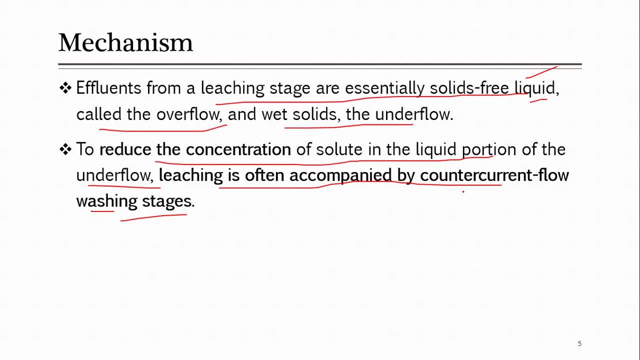 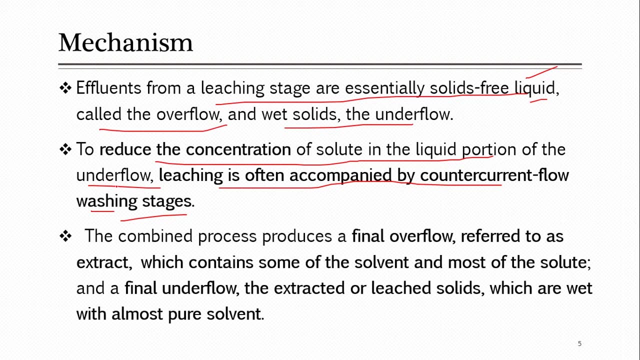 like these washing stages are somehow something similar like what we do here in, like sukkiesing of this tea bag when we are taking away it from hot water So that we can recover maximum liquid part as well as that solute which was part of the liquid. 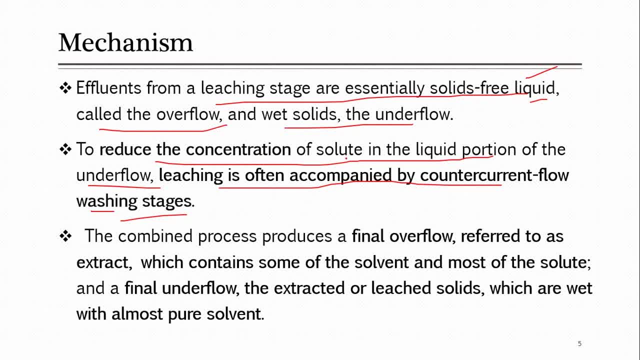 So the combined process overall, like you will have leaching stage and then washing stages if there are number of stages, So at the end combined process produce final overflow referred to as extract- I mean when you have more than one stage- is definitely this overflow will take place from one stage and it will then go to the next stage and 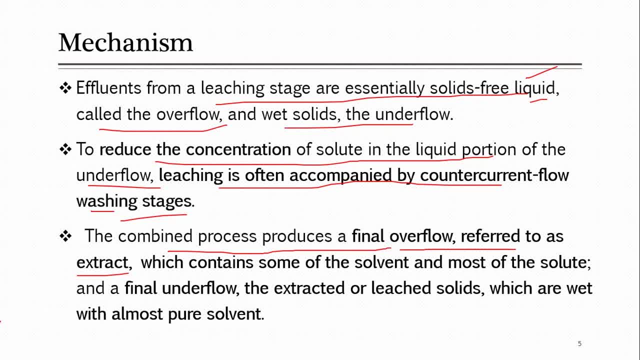 then it move and jump to the next stage and so on, So at the end when it leave from the last stage. So it is called like extract and which contain extract. you, extract is that component which is overflowing, and overflow, you know, overflowing is that which. 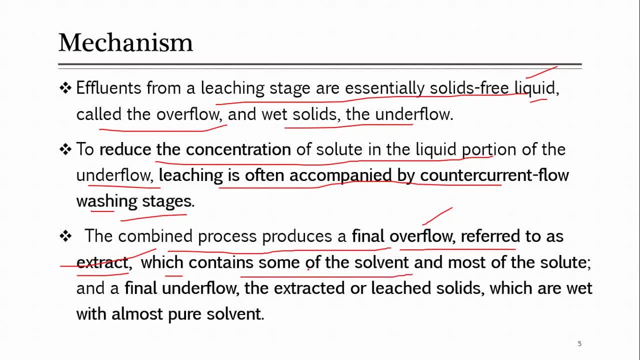 is the liquid or a solvent, So which contains some of the solvent and most of the solute. So this stream, overflowing stream, is the your solvent containing part of the solute with it. So that is named as extract here now and the final underflow, the extracted or leach solid. 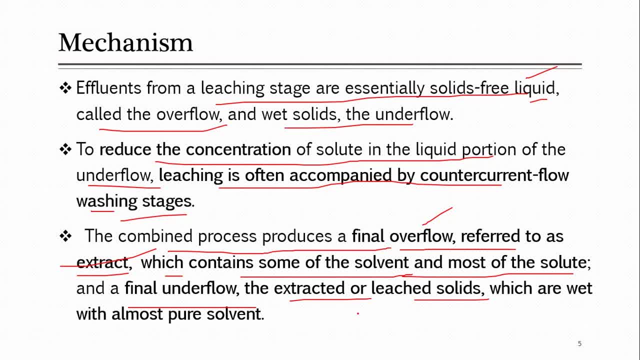 underflow are mostly the solids and they are like extracted or leach solid, because we have extracted some of parts of those solid and these are most of the time wet, which are wet with almost pure solvent, I mean that solvent which was added, So that will be somehow part of the solid and 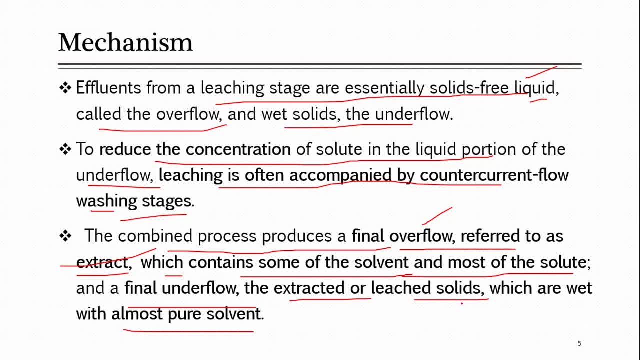 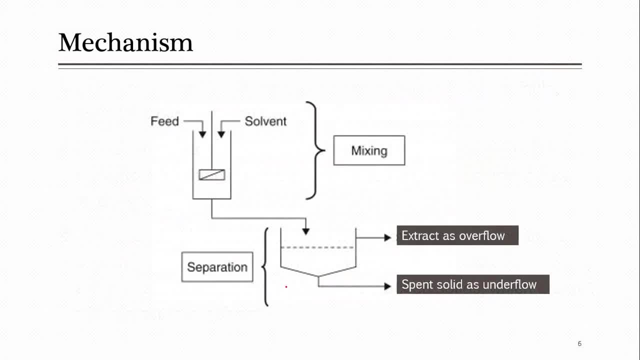 these are the extract Extracted solid which will be leaving from the last stage. So at the end of the day, this underflow which leave from the final stage is named as extracted or leach solid. So this is the one of one stage, for I mean this leaching is shown to you here overall. you can just see that. 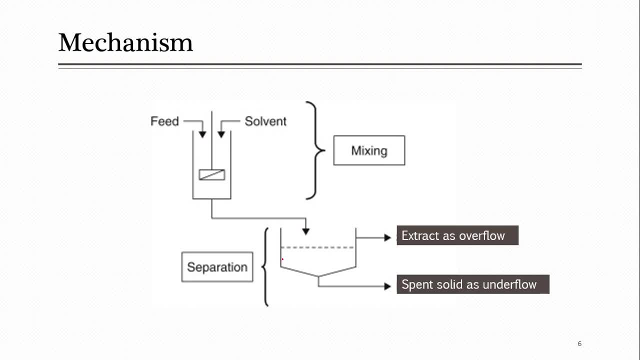 there is one stage in which mixing is taking place and then there is separation, Why we will look at this. for example, you bring in the feed here as well as the solvent. So in this phenomena in industry For leaching you have to mix them up. So you usually go for some mixing part, some impeller type. 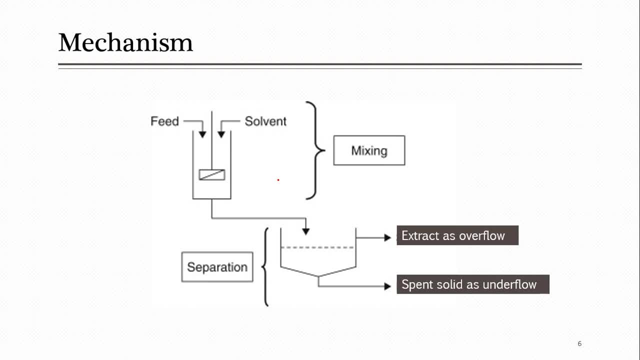 equipment to mix those. Why? so that maximum mass transfer and extraction take place. So after this you just bring it or give some settling time. So for settling you just put it to a basin which will give separation at the end based on the gravity, because solid will settle down, it will go down. 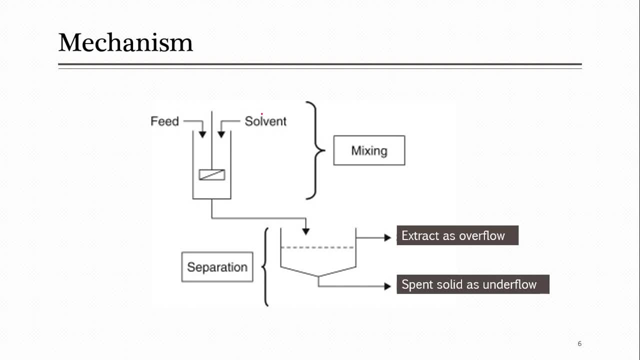 and liquid will be extracted to the top Now, because the purpose of this solvent was to extract some part of the feed. This feed is in the form of solid, So some part is extracted and becomes its- I mean part of the solvent. So this will 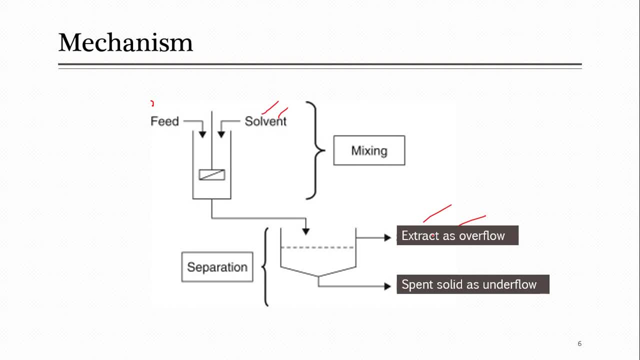 be like solvent as well as some solute and thus leaving as extract as a flow overflow. as we have seen in the last slide, extract will consist of solvent as well as salute. that was extracted, the from the solid And then the bottom portion of this are underflow, that is, the spent nivel part. Next, to contain all of these pieces, it has to be extruded totally. That means not one or two components end, not two components, and this is a lineal of which between the mallet is resulting. So you can see the solvent flow network here, equal to the брadley line as level, with length cascading up. So the check and even if we rather doocodemjan sites in meandering, coming from algorithm 1 as half, this will be. 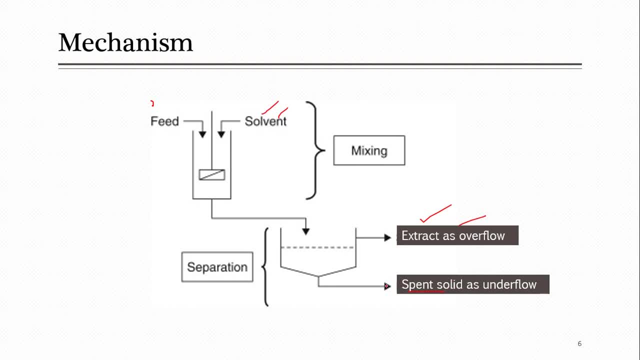 flow, that is, the spent solid. spent solid or which we called as leached solid. This is wet usually, and it contains some part of the solvent as well as there is. I mean extracted solid, I mean- which is now deprived of those solute. This is one state. suppose you have next state, so both of these will jump to the next state. 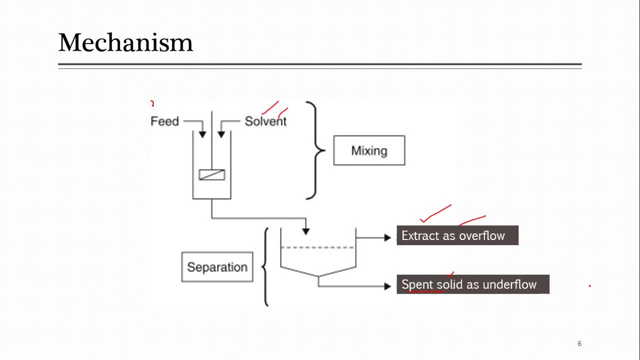 they will again come in contact with each other and more separation actually take place, and so on. Actually, not separation overall. we say like here, now, this spent solid, which is wet solid, that will contain the liquid. Now, when this liquid or solvent is leaving with this, that will contain some part of the solute and in order to recover that solute, 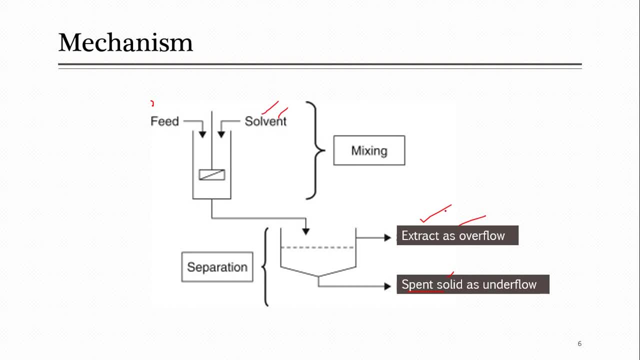 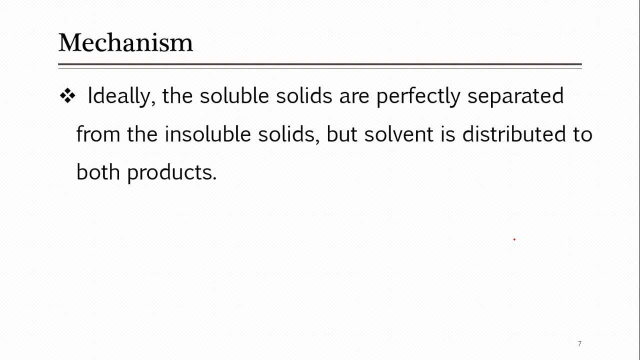 we will again bring them in contact and we will try to get as much extract as possible. So ideally the soluble solids are perfectly separated from the insoluble solid. I mean those soluble solids, the part of the solid, which are soluble in the solvent they are. 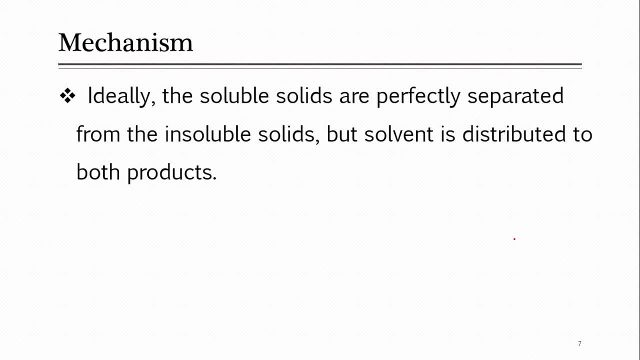 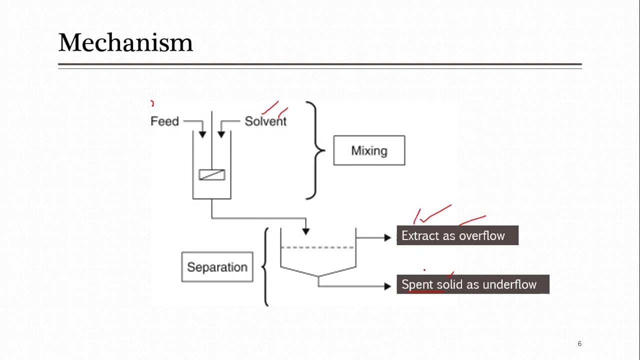 perfectly separated mean you can get even 100 percent separation from the insoluble solid part, But solvent is distributed to both products. So what does this mean like? here we have seen that the solvent which was introduced here, that is part of the extract, as well as this, under flow stream, as well as overflow stream, So that is actually is. 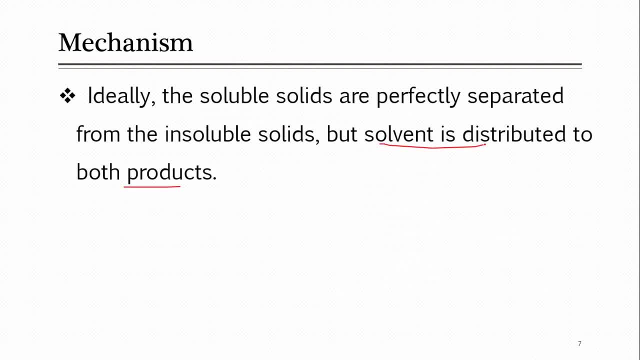 naming it here like that, distributed to both products. I mean overflow and as well as in under flow. it is distributed among both. While under flow will contain most of the insoluble solid- all of the insoluble solid, even- and top stream will contain, or overflow will contain most of the soluble solid, but some will also be. 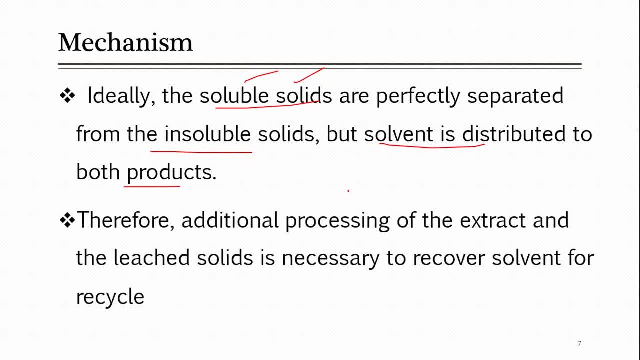 part of this. I mean under flow stream. Therefore, at the end of the day, now the solvent is usually expensive and you have to recover it. It is not like waste. So there you will have another equipment in which, at the end, you will just separate. 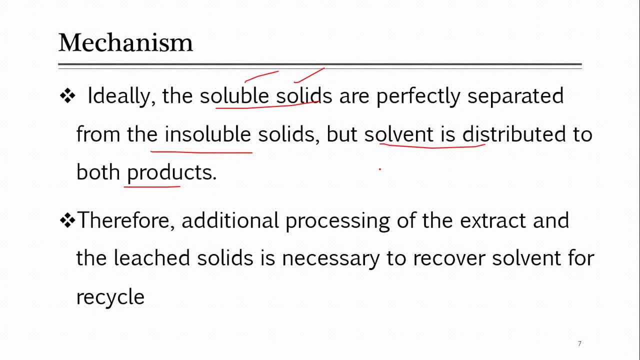 the solvent from both of these soluble as well as insoluble solid. So due to this, we say like we have additional processing of the extract and the leach solid Extract, which was the top layer, and the leach solid, which was the bottom layer, as under flow. So they 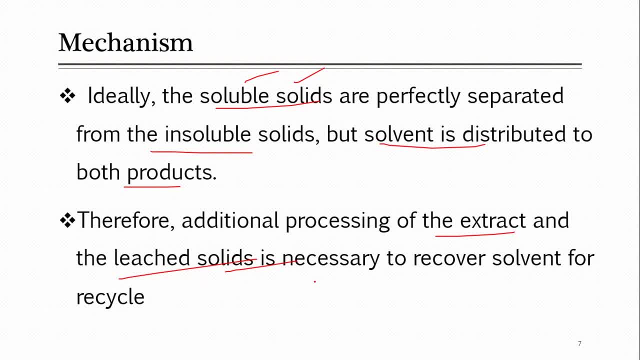 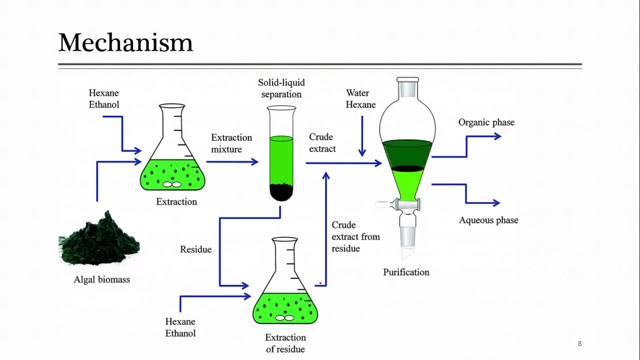 go necessary, I mean for some necessary processing to recover solvent to be recycled. So this phenomenon, So the mainitter which is the siloed, for example, here you can see like we have hexane ethanol, that is the solvent which is introduced with this algae, biomass. so you just bring them in contact and when you are, 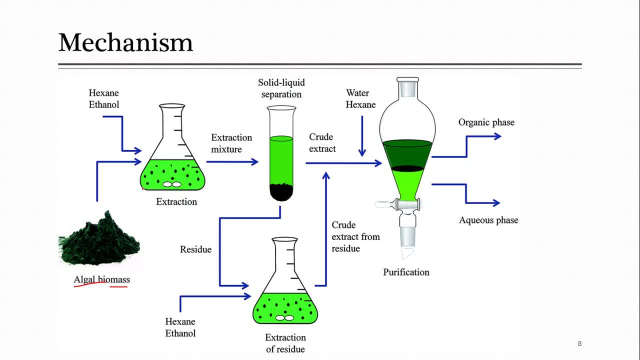 bringing. you are extracting here. Here stirring is taking place. this is the sign of stir. so just after stirring you will extract some part of this. I mean biomass that is transferred to the hexane, because these controlling So 16, the oils which are extracted, So those will be extracted to these main hydrocarbon hexane. 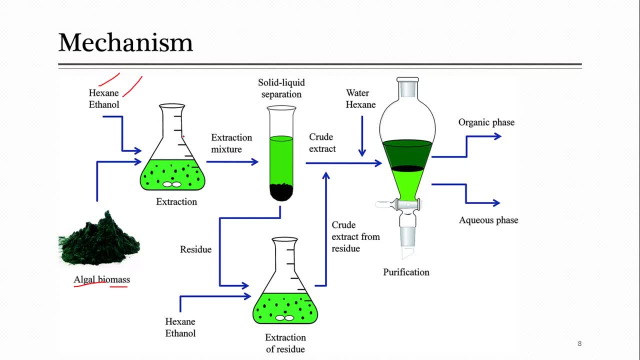 ethanol. So after this, now you have to. this is the first stage, like we have seen in the last slide, first stage of extraction is mixing. So here mixing takes place. after that you have to give them some settling time. So you just bring it to some settler and here again density base. 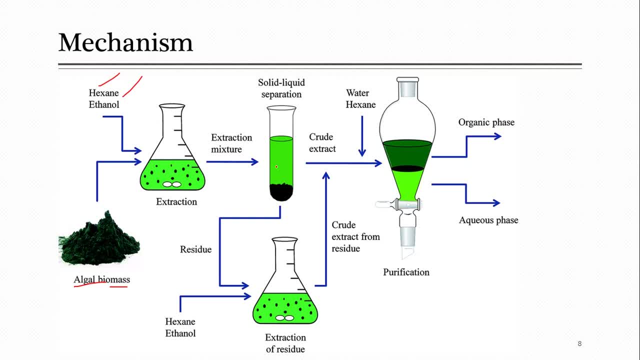 separation always takes place easily because solid has higher density and that will settle down, while liquid is at the top. And then at the end of this, I mean this solid along with some liquid leave as a residue from the bottom, and from top you get this. I mean crude, like here he is. 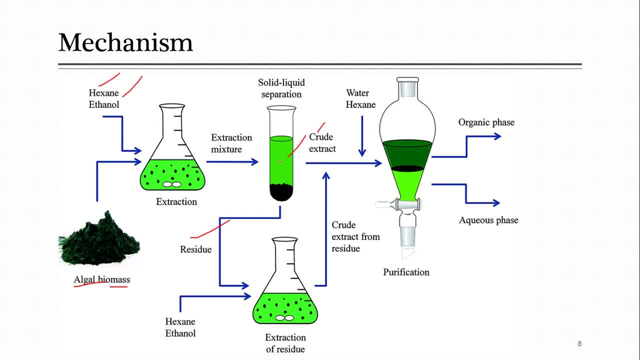 naming it like crude extract. top layer is extract, So simple. you can call it like extract, So extract. and this is bottom layer, which is spent, solid or residue. So after next stage, like, for example, this is the last stage of extraction. So after next stage, like, for example, this is: 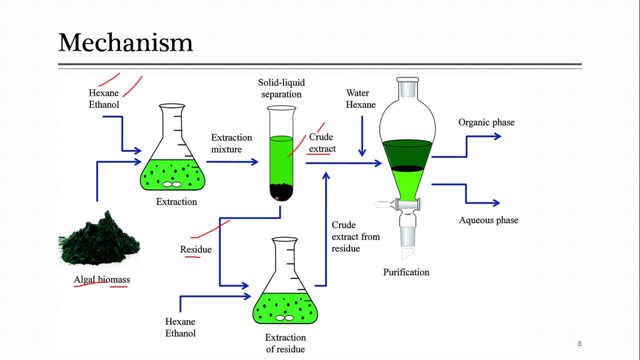 the solid residue, as you know that that contain some of the liquid and that liquid or solvent, which is part of this, will contain those oils which you were looking for. So in order to recover more of those, you go for this stage. In next stage, you bring it this in contact with some. 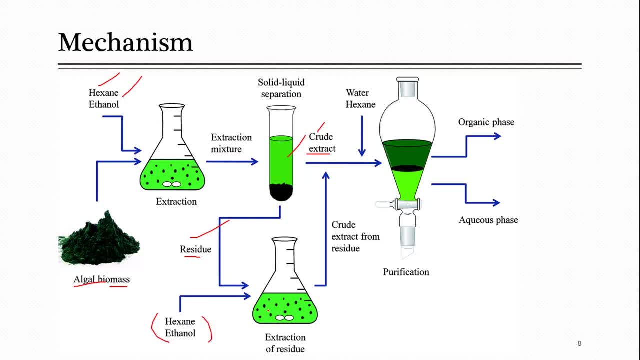 more solvent. So when you will bring it some in contact with the more solvent you will be able to extract it a bit more. This is the same similar stage like here. I mean mixing takes place. So again you will have some stage like this, which will be like somehow separation stage. So 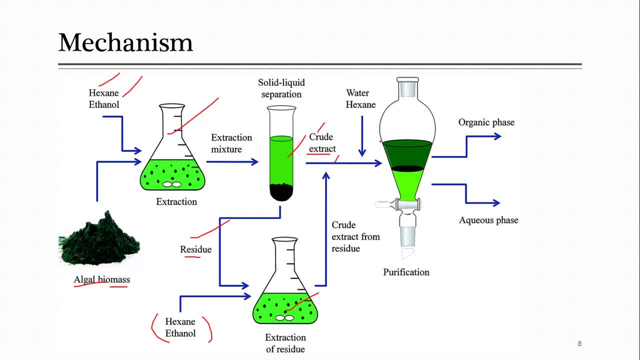 after separation stage, top layer extract to where meets with this layer and they go to the next stage. while this solid will be now final, spent solid will be removed from the system, which he did not show here. So next now process is actually to remove the solvent to get separated. 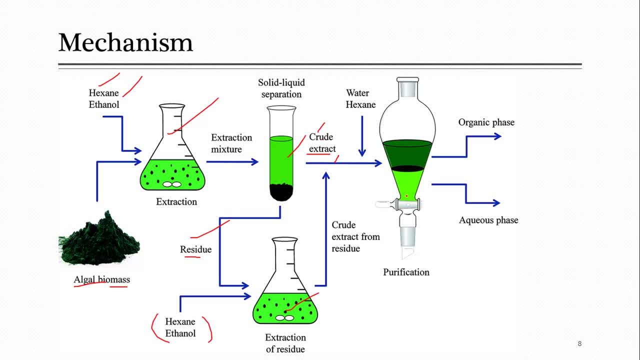 the solvent. So what you will do, just bring this extract to some separating funnel In which you give it some time. So after for some time it gets separated to 2 phases. I mean, it depends on the application. sometime it is not only like this simple settling. sometime you 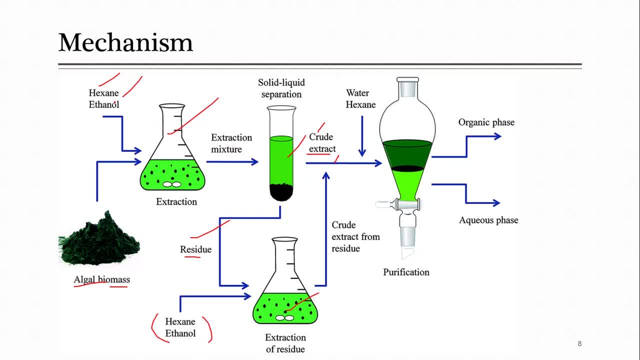 can just get separated these chemical like extracted and the original solvent, with the help of distillation, some other separation technique. but you will need some separation technique just to get them separated. So when you get them separated later solvent is recycled here other product is obtained. So this is all about the mechanism. 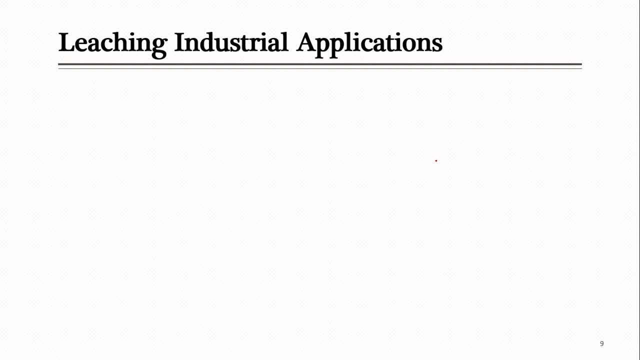 Next, like now we know that this solid liquid extraction is used in the industry. So what are major industrial application like? initially we saw that it is used for metallurgical, some food industry. So what are major application where it is used? So industrial application. 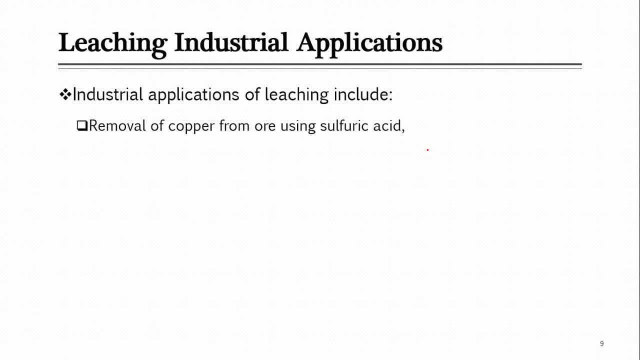 of this leaking include, first of removal of sulfur from sorry copper, from the ores, using sulfuric acid. So sulfuric acid here is a solvent and those ore is a solid. you know that ore is a mixture. I mean that is not only the copper, the. it will exist in the form of. 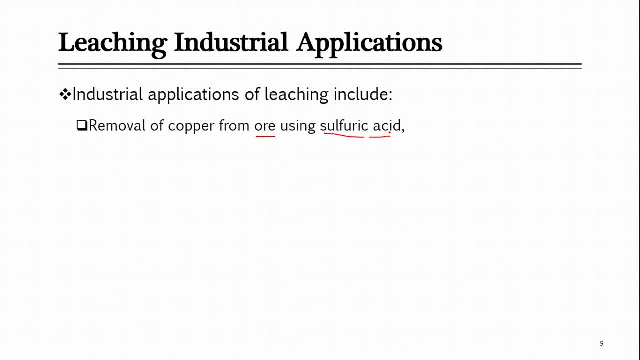 some other chemical, like may be carbon nitrate- carbon I mean sulphate or I mean various different salts- are possible which are extracted from the mine. So in order to separate that, specifically copper, from this, we use sulfuric acid. So sulfuric acid will be used to extract the copper from the mine. So in order to 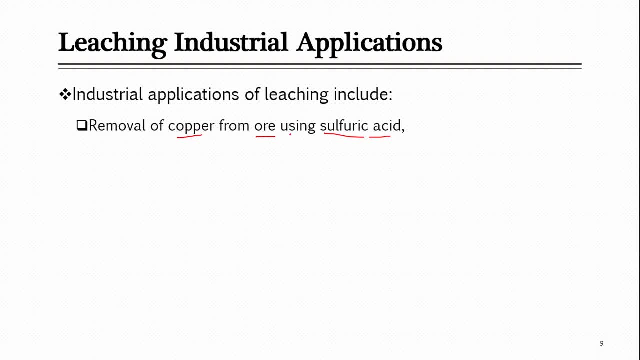 separate that, specifically copper, from this. we use sulfuric acid. So sulfuric acid will extract from that ore only the copper and all other is left as a spent solid. Then recovery of gold from ore using sodium cyanide solution. So this is used for recovery. 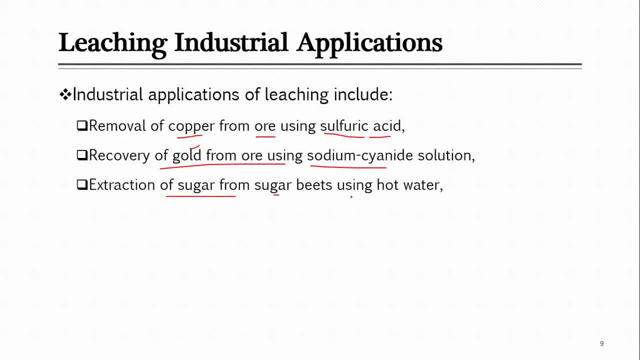 of gold. Then there is extraction of sugar from sugar beets using hot water. So this is different example as compared. whether So this is, this will be example of food industry, in which what you are doing, you are extracting the sugar from sugar beets by using hot water. 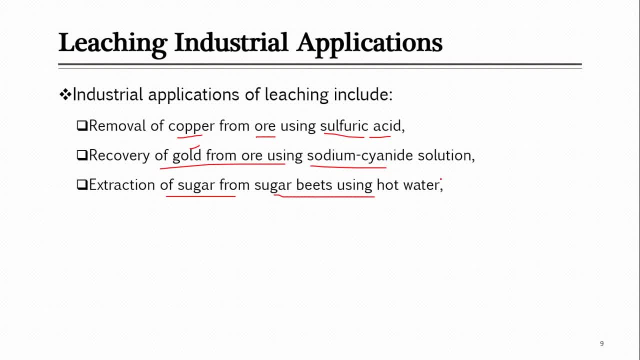 So when you bring them in contact to the hot water, So when you bring them in contact to the hot water, Hot water extract the sugar from those sugar beets and then solid residue is left. Extraction of tannin from the tree bark. 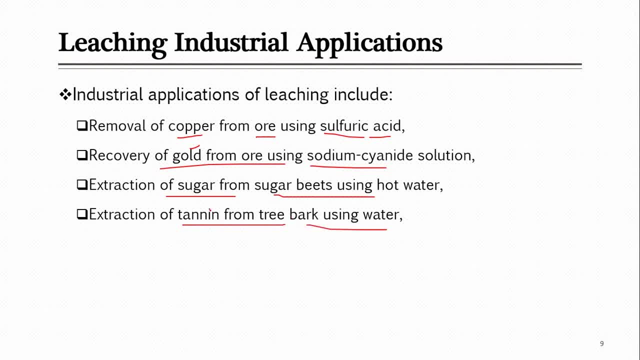 using water. I mean removal of tannin from tree bark using water, just another example mean. Then there is removal of caffeine from green coffee beans using super critical CO 2, or even you use. I mean they extract this coffee caffeine from the coffee with the help. 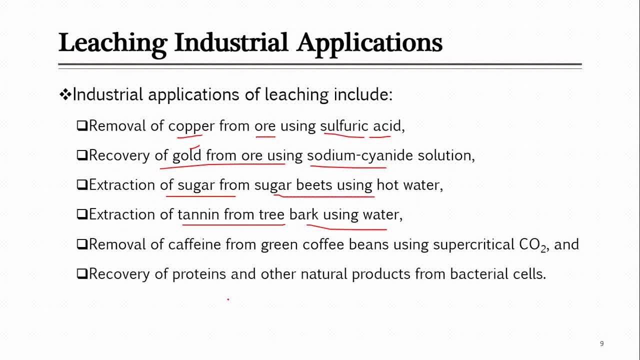 of hot water. So that is application from food industry. Then recovery of protein and other natural products from bacterial cells. So this is somehow mean the application of, you can say, overall biochemistry side application. So these are the various leaching application. 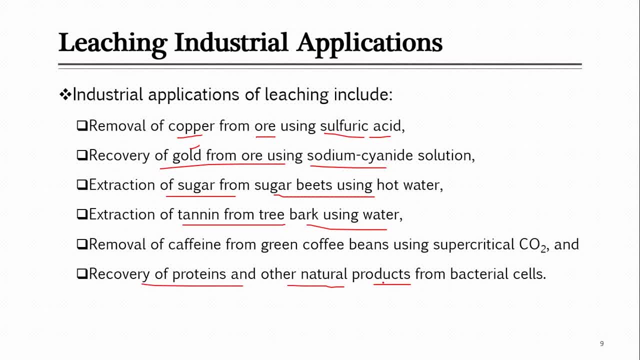 which, on in which leaching is used for extraction of various components. And in all of these application, your feed will be a solid, like these will be: or there is a sugar beet, there is a tree bark, So all these coffee beans, So all these are the solids. finally, and you 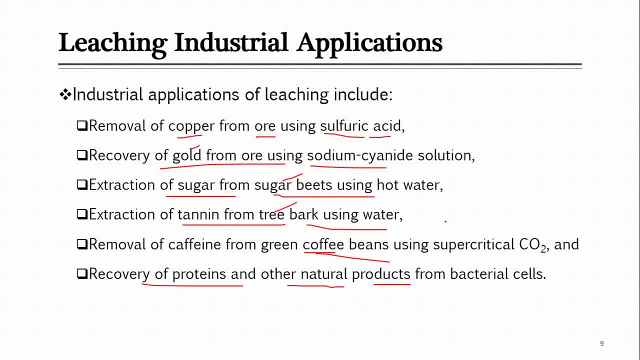 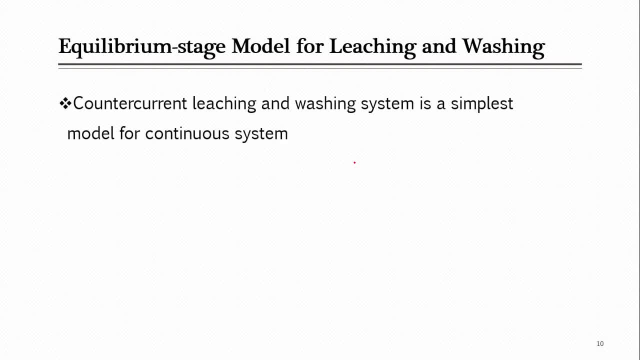 extract them with the help of some liquid. So all liquids are described here. So next then the- I think last part of this lecture, which is about equilibrium state model for leaching and washing, As I mean two, three slides back. you remember that We decided. 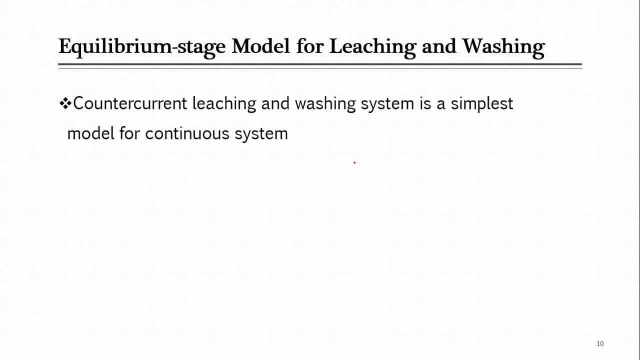 discussed that most of the time there is leaching and then washing stages. So this model actually discussed those that phenomena of leaching and washing. So let us look at this in detail. equilibrium stage is called equilibrium stage model for leaching and washing, and sometime 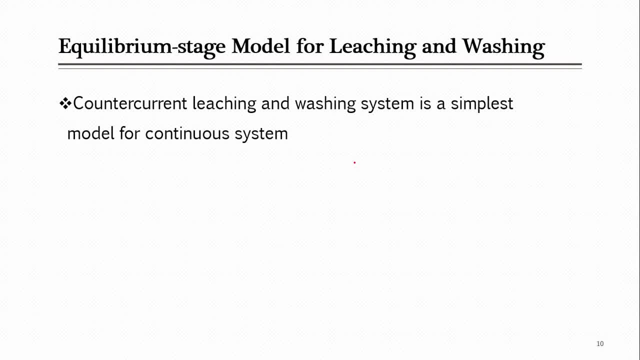 also named as counter current washing method. So in this method, actually what you do, this in counter current leaching and washing method or a system, is a simplest model for continuous system when we describe the continuous leaching system, leaching and washing system. So this: 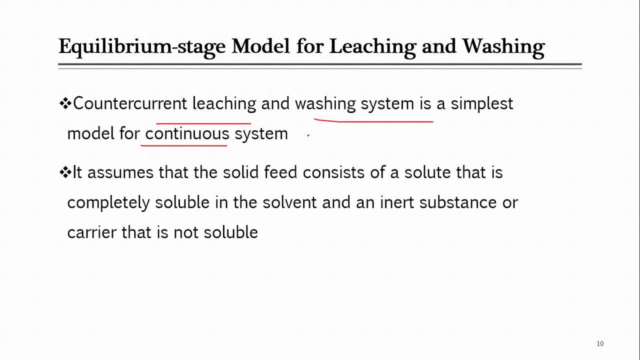 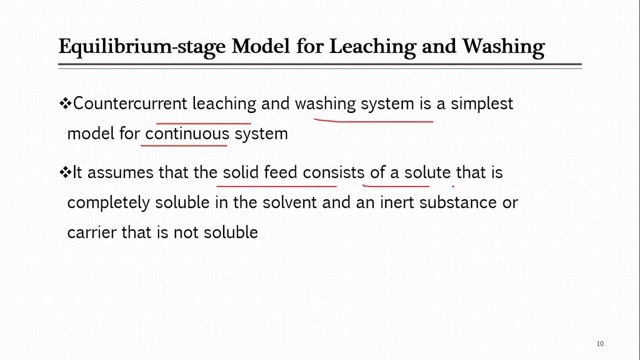 counter current model is the best main model, which is the simplest model and used mostly for main discussion, for design, for calculation. So it this model assumed that the solid feed consist of solute that is completely soluble in the solvent. I mean this is considered that I mean solid feed contains some portion which is called 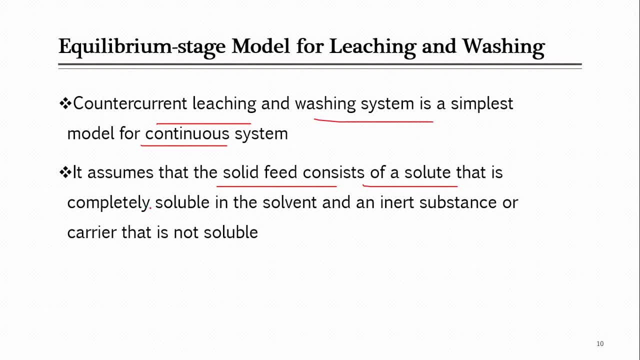 solute or leachant. So that is soluble, completely soluble in the solvent. you bring it in contact with some solvent and it will completely dissolve in that solvent, while inert part or inert substance or the carrier is not soluble. As I told you, like solid will consist of two parts similar, like the liquid, liquid extraction. 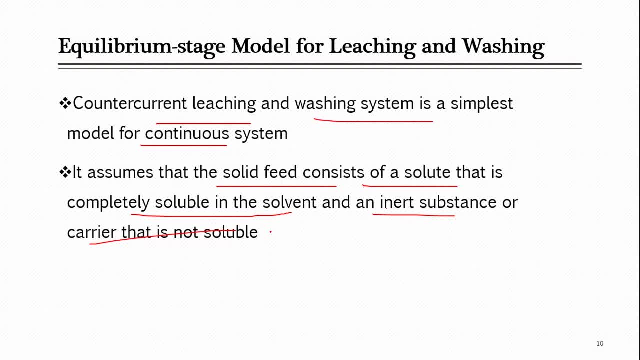 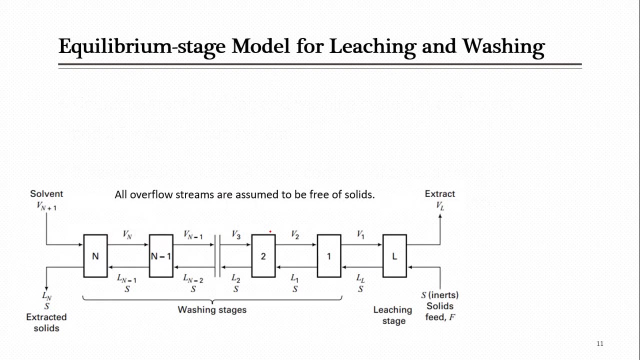 like in the liquid, liquid extraction. your feed consist of liquid that contains some parts which can be extracted with the help of other liquid and some just stay as such. So here again means solid consist of two parts. one part is soluble in the solvent, while other part is not soluble, So that is we call it like inert substance or the carrier. 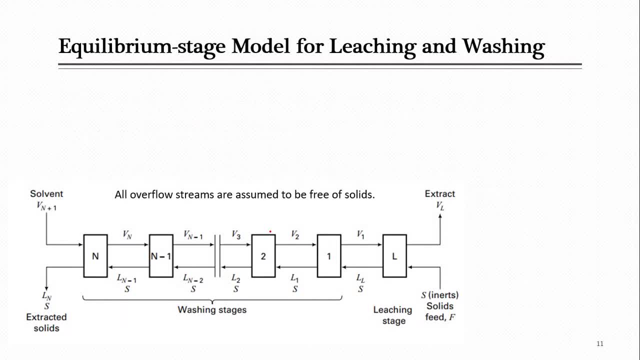 Let us look at this. So this is the- I mean leaching and washing, counter current, I mean counter current model. So in this, just look at the diagram. first of all, here, this is one stage, leaching stage. I mean you have leaching stage and, as you remember, we said: 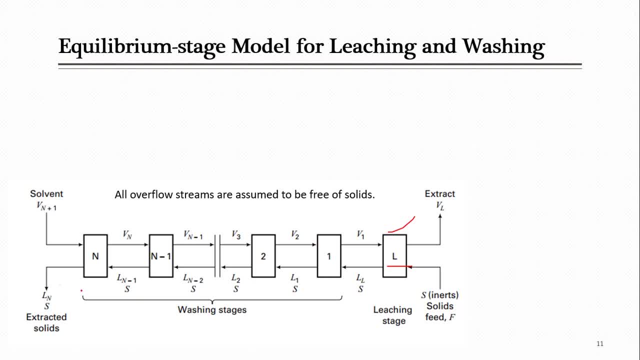 that usually leaching stage is only 1 stage. then there are other washing stages And I told you already, but again here I will discuss this point- that why you are looking for the washing stages. So what a? in this stage you can see that. 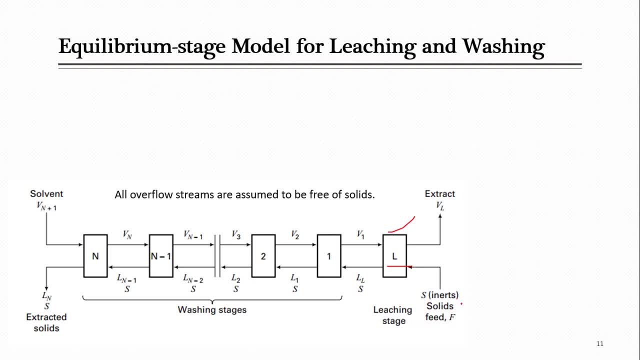 that there is some s inert solid solid feed overall. just, I will just define these s f. what does this mean? different terminologies here are mentioned. ok, just let us look at them. s s is the mass flow rate of inert solids constant from stage to stage. just think s mass flow rate. 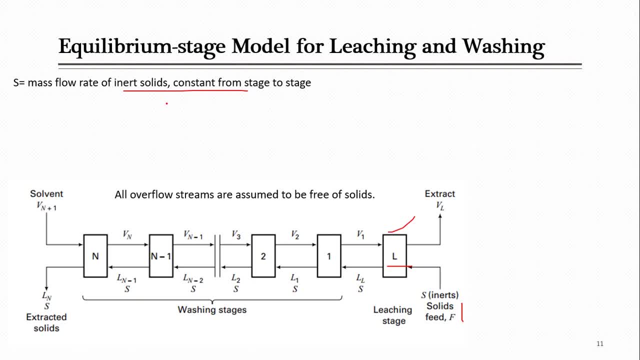 of inert solid because we said our feed will consist of two solid parts: one is soluble in the liquid and other is inert carrier. So when we are saying that is insoluble, So it is mean it will remain constant throughout all the stages due to this just represented. 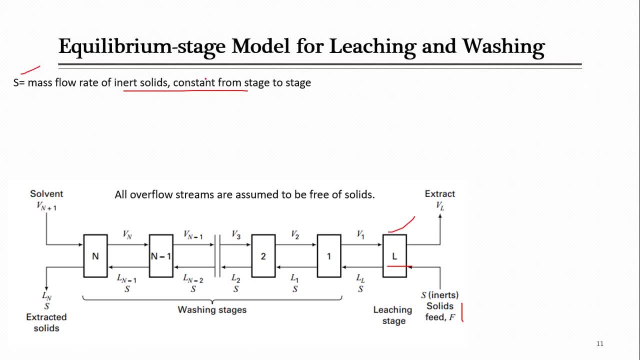 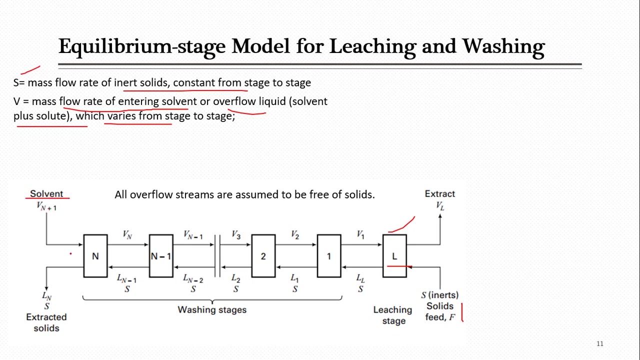 with s simple mass flow rate of inert solid, which is constant throughout the stages. Then there is v other v I mean v indicates mass flow rate of entering solvent or overflow, liquid solvent plus solute which carries or which varies from stage to stage. So here you can see this solvent which is entering at n plus 2, n plus 1 stage. So we 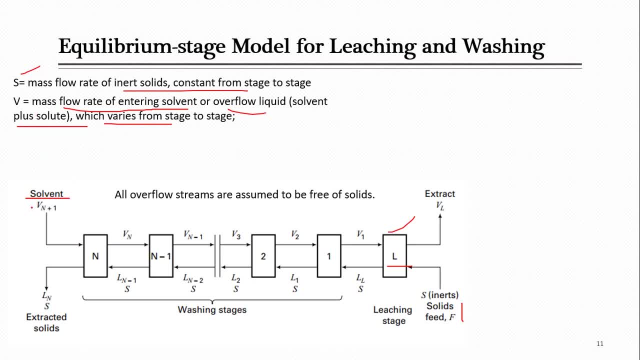 will talk about these number 1, 2 and later. but just consider this: v is entering, which is pure solvent at the start. but as he said that this will be the pure solvent, but later on, because this solvent extract some part of the solid, So this will be later becomes. 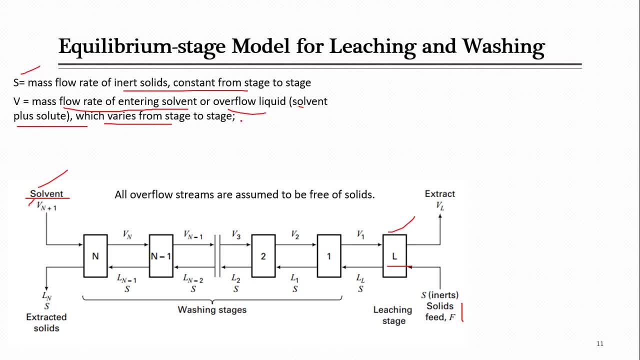 solid solvent plus solute, and I mean this v and this v will vary. why it will vary? because initially it is pure solvent, but later on, when it is passing through various stages, it is extracting solute from each stage. when it is passing, it is extracting solute and 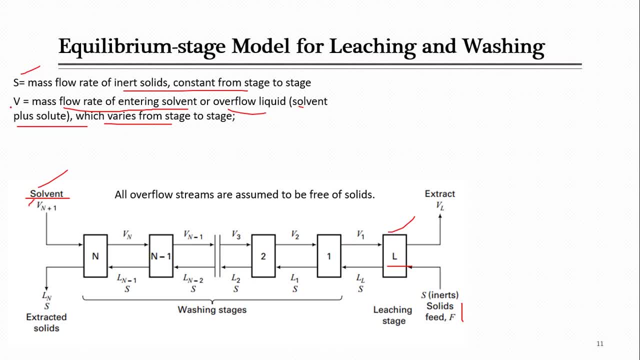 the concentration of solute will keep on increasing in this v. So due to this is composition will be. our amount will be varying throughout the equipment at each stage. Then there is also this mass flow rate of the underflow liquid, like here when you see: 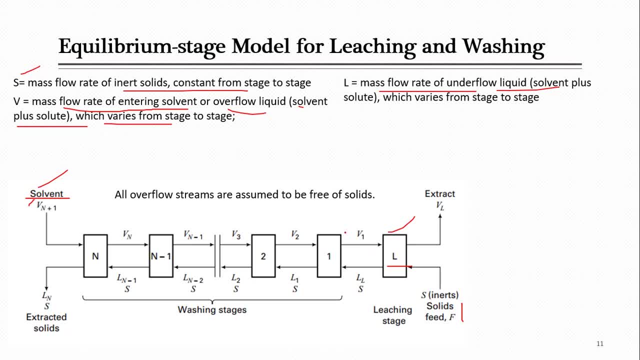 that our through each stage, there will be overflow liquid as well as underflow liquid. So this v, which was named as like entering solvent, are the overflow liquid. So similarly, we will have something called mass flow rate of underflow liquid. So here, underflow liquid. 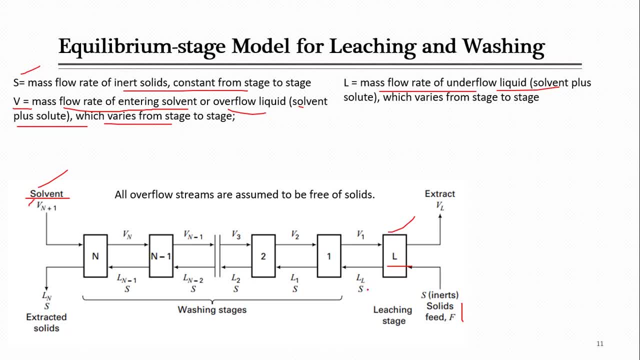 will be passing through this each stage. that will be part of actually this solid means this solid is not passed as a solid. it is wet solid, So it will contain some liquid, So its flow rate is this: L mass flow rate of the underflow liquid. 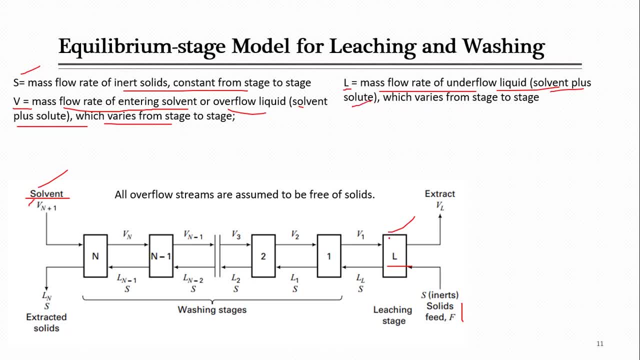 And this is usually the solvent plus solute, both because, as I told you earlier that the, when this mixing takes place, the liquid which is separated as a overflow as well as underflow, that will contain solute. So both of this, even overflowing liquid as well as underflowing. 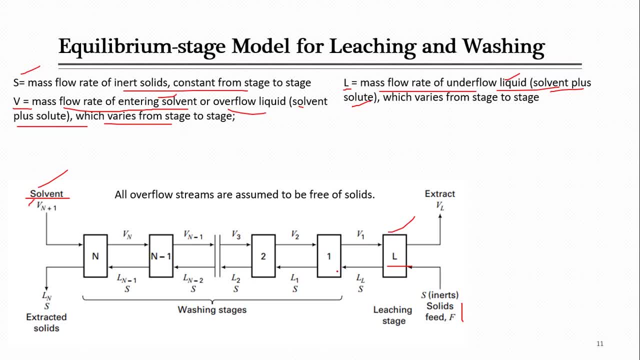 liquid will contain some part of the solute. And these stages, the washing stages, we are just bringing these stages because we want to reduce the amount of this solute which is being carried out in these stages. So, overall, when you will just keep on moving from here, stage 1, towards n amount of this, 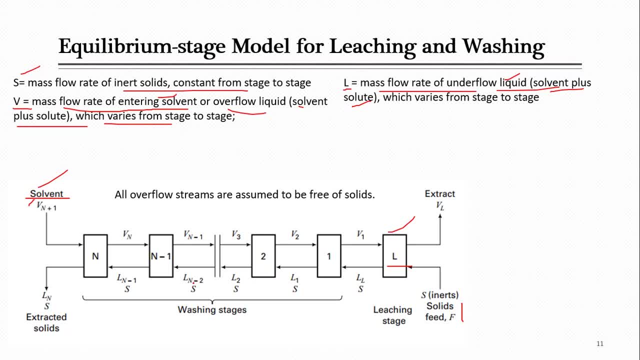 means solute will keep on decreasing inside this underflow. why? because we will be extracting it in each next stage: towards solute, towards top layer, towards overflow. We will be extracting it due to this, solute amount will be varying And when its amount will be changing due to 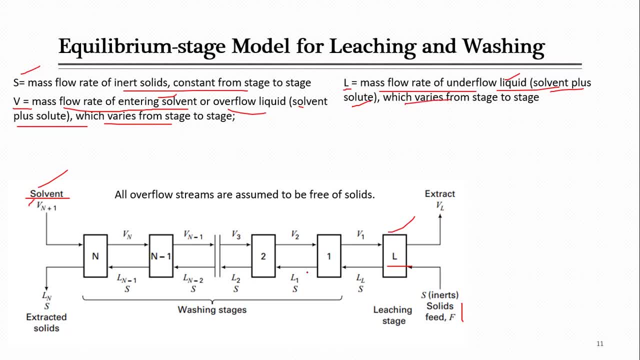 this overall. this flow rate will be changing from each stage to stage. So hopefully now you are aware that overall here we will be talking About three streams. first stream is only the solid, which are inert solid. they will stay same throughout. according to this model, actually equilibrium stage model, it is considered that 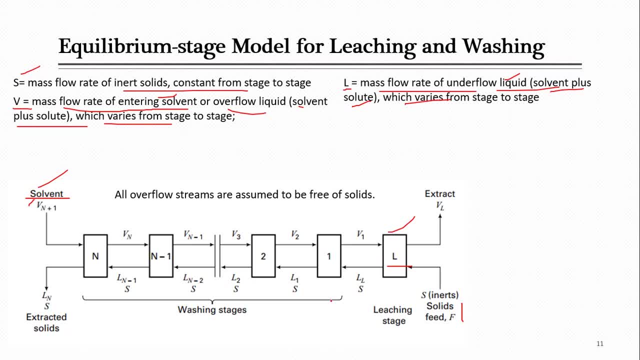 they remain same. Later on, in the next slide, we have to look at some other assumption of this model. So, based on that, this amount of solid, inert solid, remain same. And then there is V, solvent, which is entering at the. initially it will be only solvent. 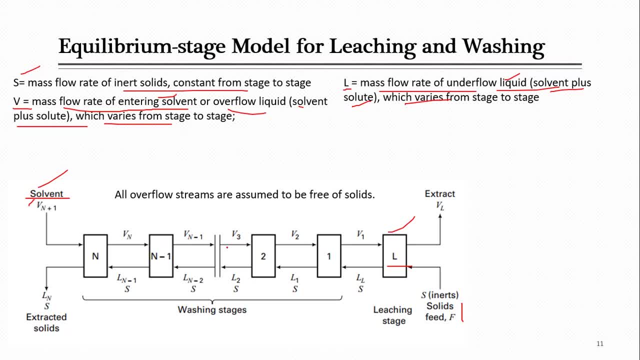 but later on it will carry the solute with it. as it will pass through the various stages, Its amount will be varying. then there is L is the mass flow rate of underflow liquid. So it initially will contain some liquid which is solvent as well as solute. but as 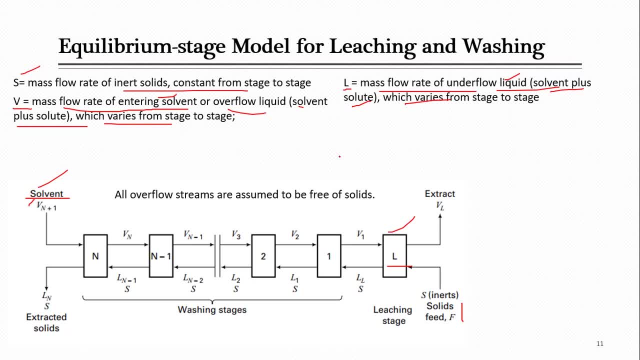 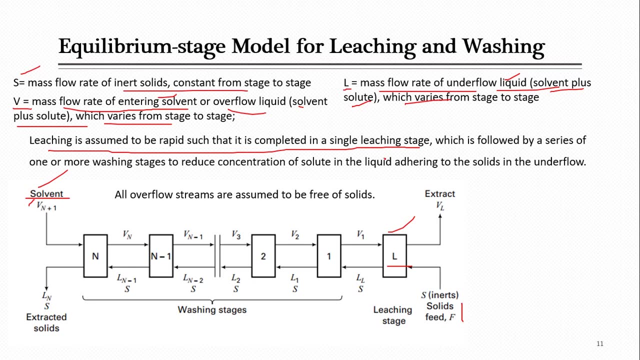 it keep on moving from stage 1 to n, we will be extracting or we will be removing amount of solute. due to this its amount will be decreasing. So it is assumed here leaching Is assumed to be a rapid, such that it is completing in a single stage, even like leaching can be. 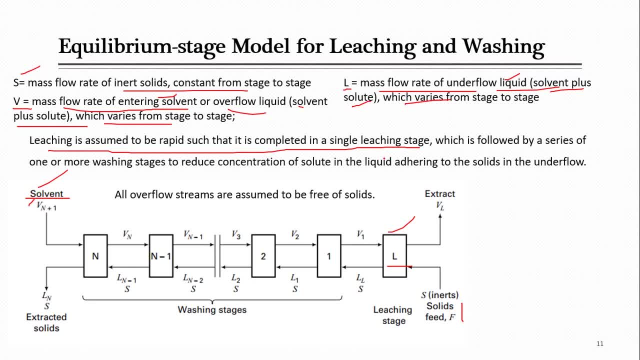 completed in a single-stage. The solution under flow ratio depends. like it is single stage, you maybe don't need more than one stages, only in one stage. I mean complete leaching. 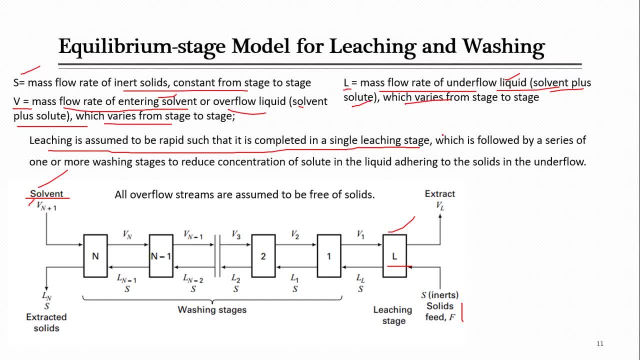 can take place, but there is a problem of this leaching. after this leaching, like in this stage, when this solid and the liquid came in contact, part of the main solid was extracted. that became solute. solute become part of the main extract layer. but when this wet solid is leaving, so that 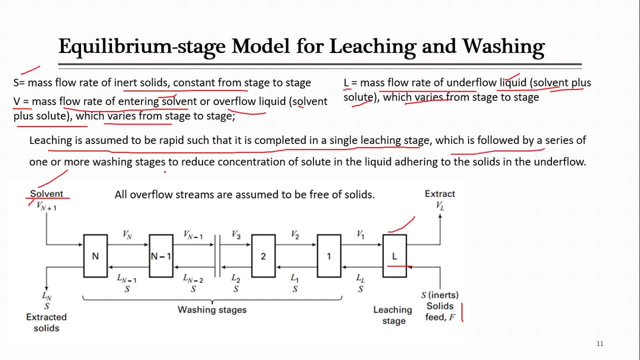 contains some amount of solute. so this leaching stage is followed by a series of one or more washing stages. why those washing stages? washing, as its name indicate, you are washing something. what we are washing, actually, we are washing the solute as it keep on moving from these stages to 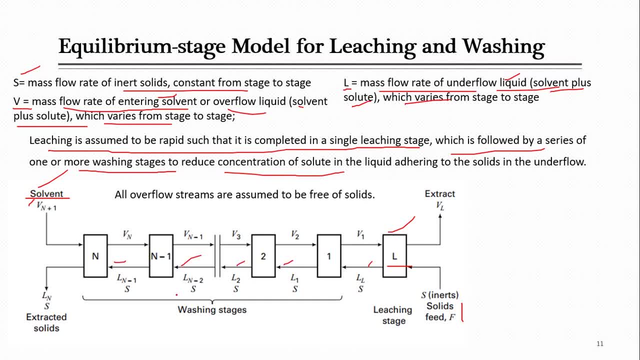 the next stage we will be removing the amount of this solute from this underflow towards main overflow. just use for removal or reduce the concentration of solute in the liquid. adhere to the solid in the underflow because this solid can't be only the solid. it will always contain some liquid, because solid has tendencies to carry liquid with them. 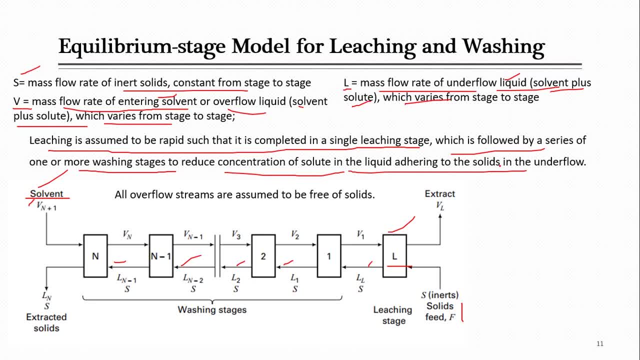 so when this liquid is being carried, we will try to extract as much solute as possible. due to this, you have a lot of like here, stages which are called washing stages, and like why here indicates I mean later on in the formulas it is used. so why is the mass fraction of the 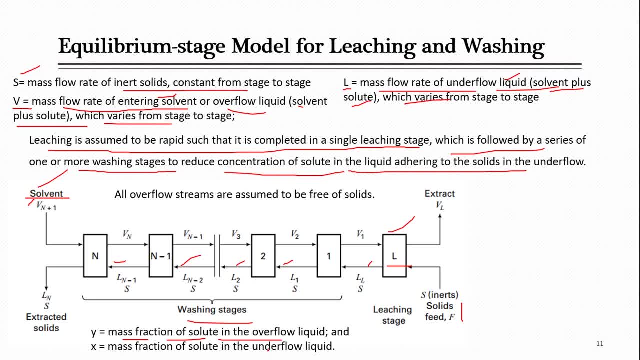 solute in the underflow liquid, while x is the mass fraction of solute in the underflow liquid. if I tell you, initially y will be small here. y will be small initially when it solvent enter, even y is 0, but it y will keep on increasing in this direction. y will increase and x. x will be highest at the 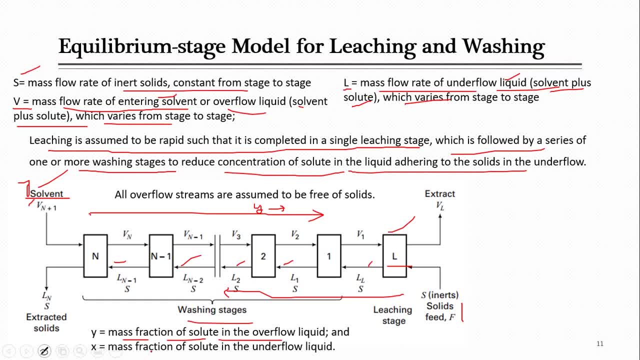 start, but later it will keep on decreasing because x, he said, this is the mass fraction of the solute in the underflow. so initially it will be maximum here, but it will keep on decreasing as you keep on moving in this direction. so overall I can say: 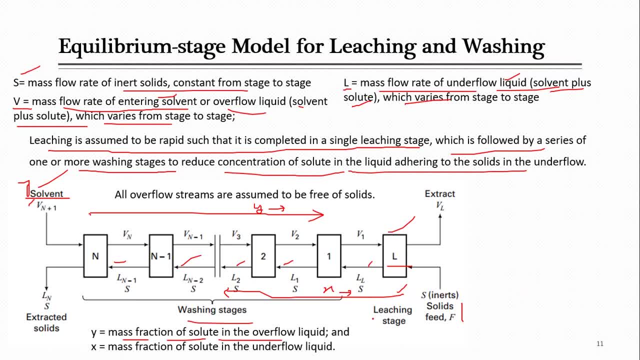 its amount will also be higher in this direction. on the right side and the left side it amount will be keep on decreasing. I mean in underflow liquid. its solute amount will be decreasing its name, like here it is just indicated with like leaching stage. then there is washing. 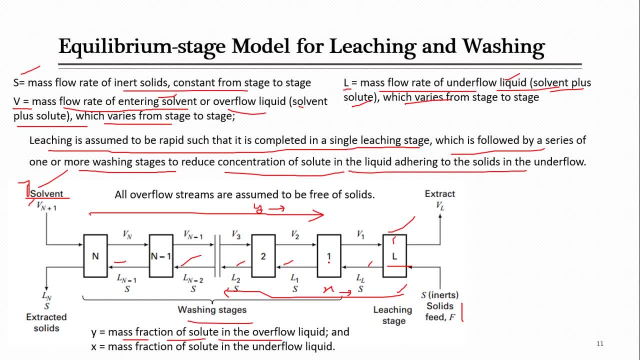 stage, so washing stages can be more than one, as we said. so like it is named first from the side from where solvent is- sorry- your feed is entering, like solid feed, entrance side is named as 1.. So after that 2 and so on. 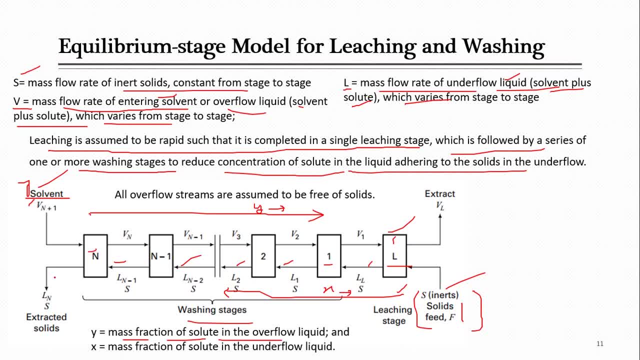 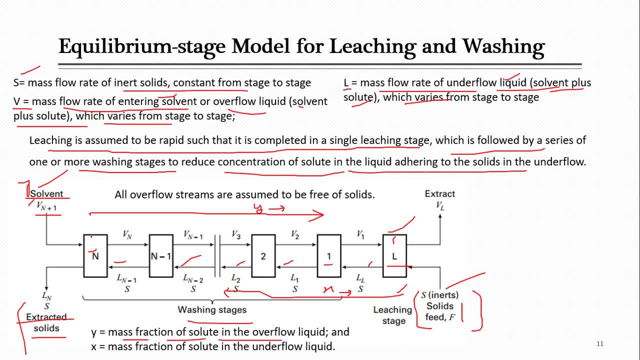 entering from n plus 1 stage, because stage after this pose n is 25, so this is coming after 25, so there is something coming from 25, 26, so 25 plus 1, and this enters. then it keep on moving and finally, from stage 1 washing stage it enter to the leaching stage and in 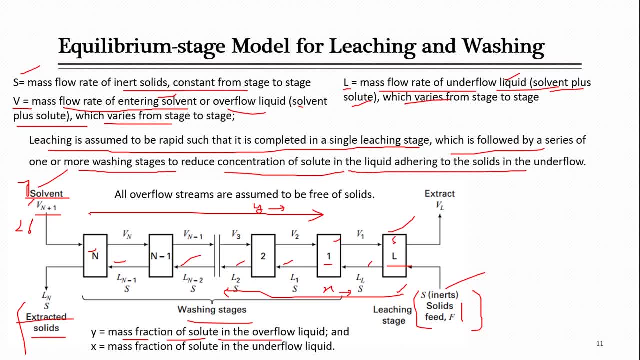 leaching stage it come in contact with this solid and then, in maximum extraction, take place here and then it leaves as a extract, final extract, liquid extract, solvent. So this is all about the phenomena here. why we call it counter current, as you can see easily that your feed and solvent are moving in the counter current direction throughout. 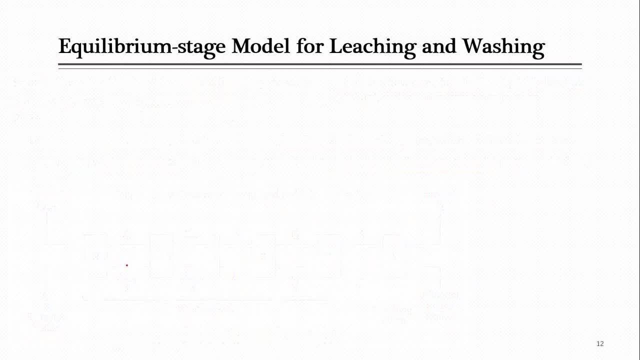 the process. So, overall this model, discuss also the equilibrium between leaching and the washing, or the leaching Ok, the washing or overall an ideal leaching or washing stage is defined when, when you look at the system in which you discuss this leaching and washing, because there will be many question. 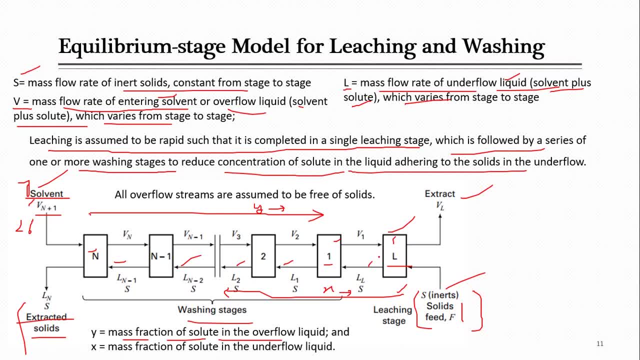 raising in your mind that it is possible, some solid, this which you are calling only inert. it can also become part of the main liquid stream and some other possibilities are there. so let's discuss those possibilities. so they are considered in this model, they are just assumed as ideally. 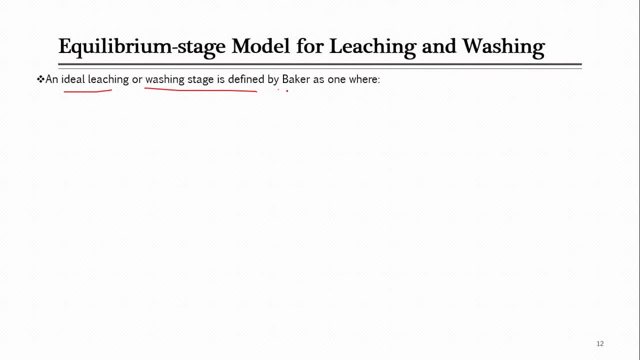 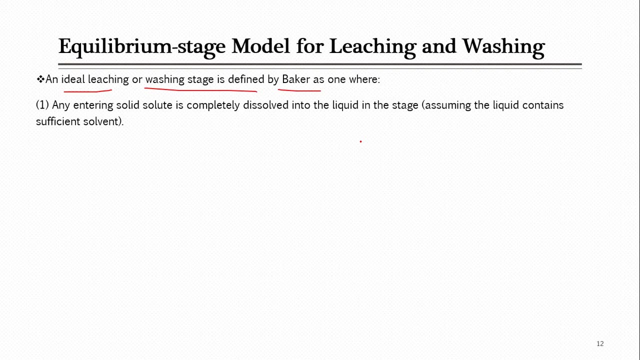 so an ideal leaching or washing stage is defined by baker- this is one of the scientist i mean who has worked on this. so he considered that, first of all, any entering solid solute is completely dissolved inside the liquid in the stage. any entering solid- sorry, any entering. 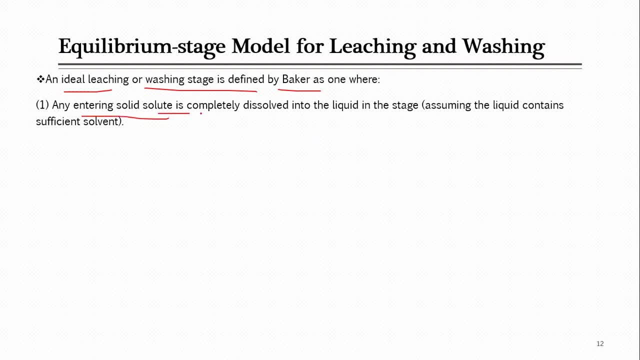 solid solute. the salutes for part of the solid which you want to extract so that is completely dissolved into the liquid in the first stage, like leaching stage in the stage mean leaching stage assuming that liquid contain sufficient solvent. this liquid which we are just bringing it as a solvent, that should be sufficient in amount when it. 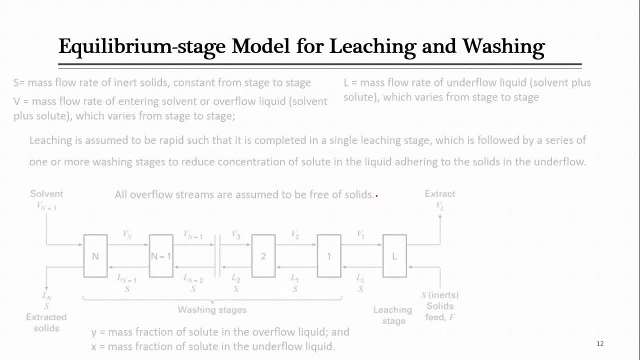 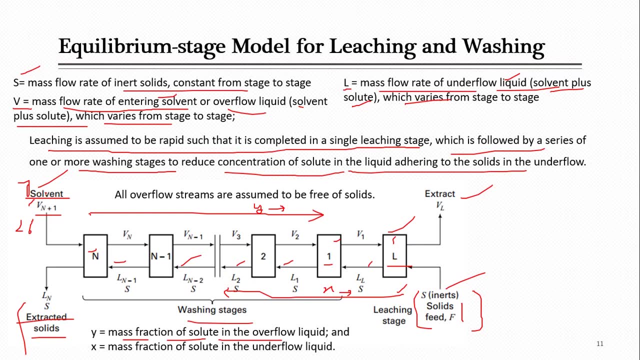 is sufficient in amount, it is considered that all extraction of the solid takes place here in this stage, mean initially, when you will start this process, just consider there will be only solvent coming here and there will be the this feed coming here. so when they come in contact in any other stage, there is nothing. 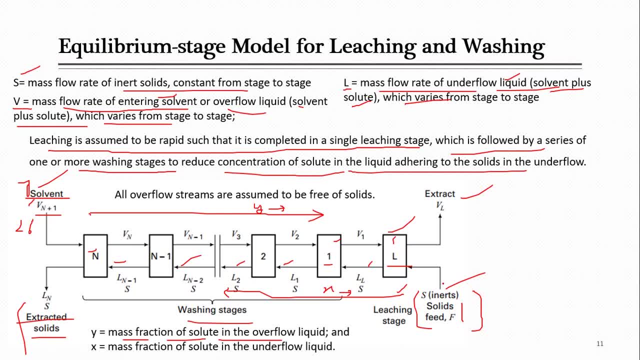 So I mean just it will pass from here directly to there and you are entering the feed when they come in contact maximum we say that all extraction takes place here. Now, after this extraction, definitely some liquid is leaving as extract and some become part of under flow with the solid. 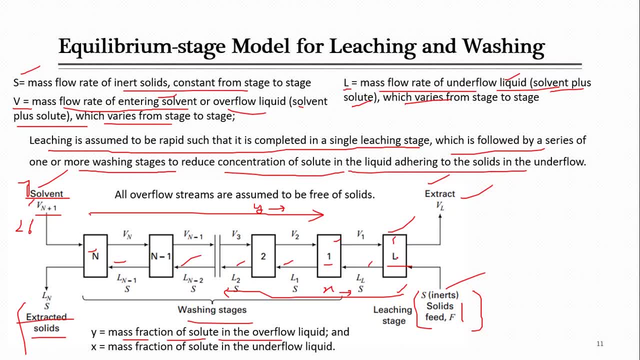 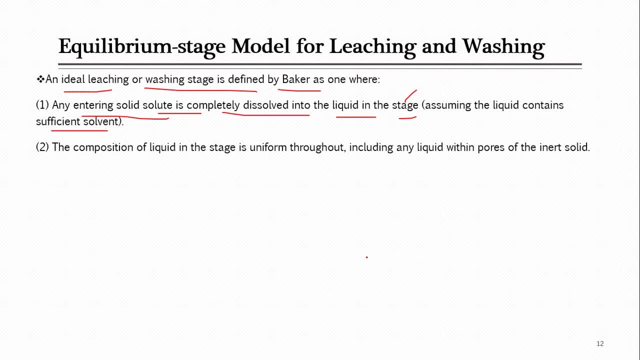 So later on in this stage some solute is carried out with that liquid, but all solid mean this solute part was extracted with the liquid in this stage. this is the first assumption. The second assumption is the composition. The composition of the liquid in the stage is uniform throughout, including any liquid. 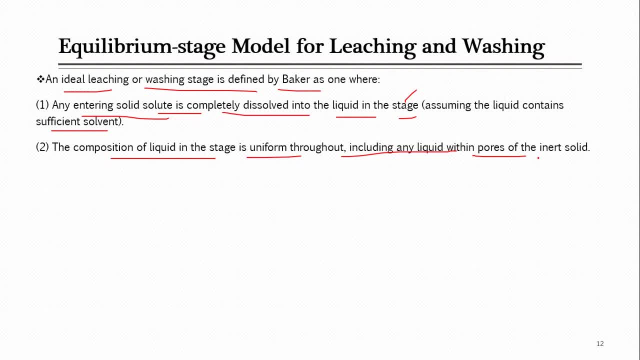 with the pores of inert. within the pores of inert solid, We consider here when this liquid has extracted the solutes. I mean from the solid. so throughout the stage, throughout one stage mean when you consider either stage 1, either I mean extraction stage 1, sorry, washing stage 1, or end stage, or I mean leaching stage. so throughout all. 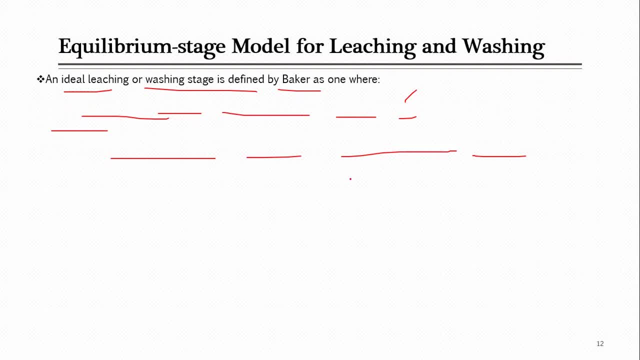 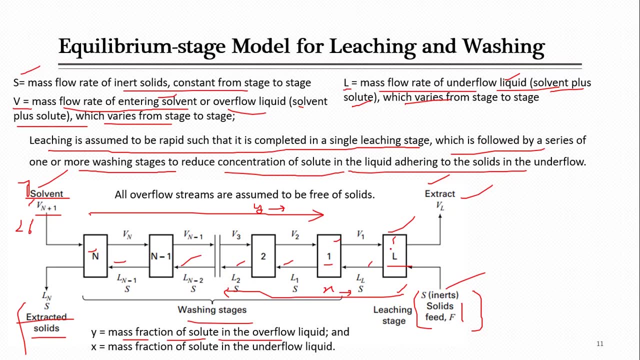 these stages? When is when you just consider only one stage. in one stage all the composition of liquid is same. Just we consider here, like for example, in this leaching stage, all the liquid which is inside. this will have throughout the whole composition. Actually, what we consider when we consider complete same composition throughout the equipment, 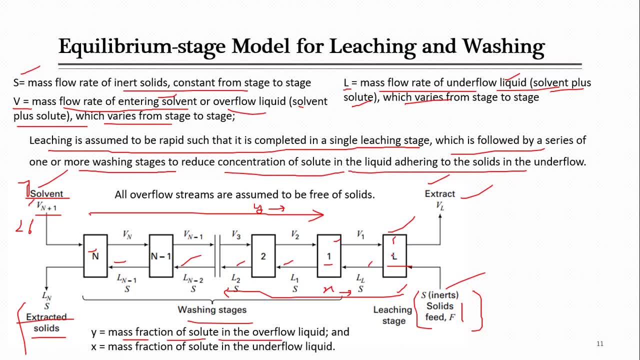 Hopefully you remember from reaction engineering that when you consider complete mixing- So this is complete mixing here- when complete mixing takes place, we consider that concentration throughout the mean unit is the solution. Ok, same. and when something is leaving from here, liquid will have same concentration as this. 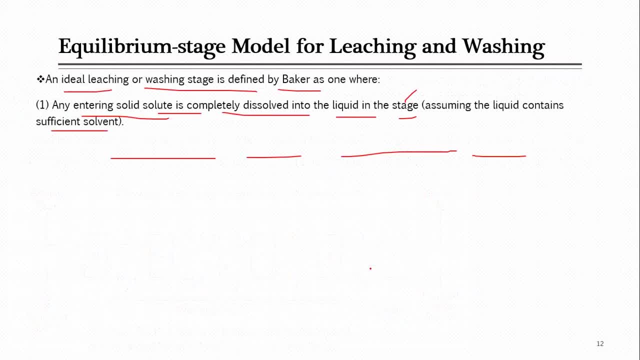 as well as under flow, liquid which is leaving will have same concentration, same composition. So composition of the liquid is uniform. but in next stage when we will go, definitely it will vary from the first stage, but that will be constant throughout the same stage. and 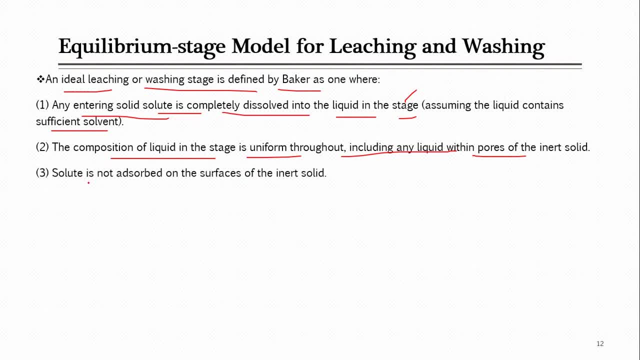 so on. I mean solute is not adsorbed on the surface of inert solid. the solute which we were removing from the solid, that is not. I mean adsorbed on the surface of inert solid, because you may think, like somehow, like when this is, I mean extracted. 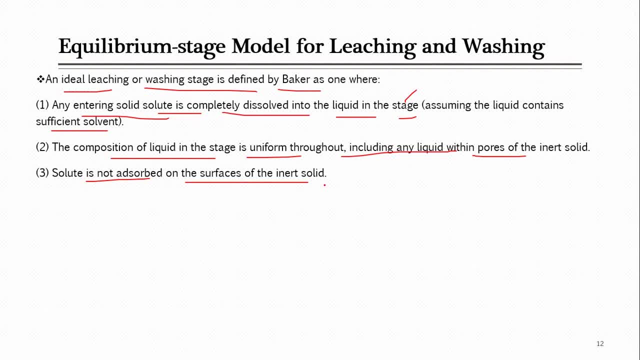 So that can become part of the- I mean- surface of the solid that can adsorbed. so that possibility is just neglected here, that it is not adsorbed. So only we consider that the solute which is- I mean these are- which is extracted from this solid that is now only dissolved in the 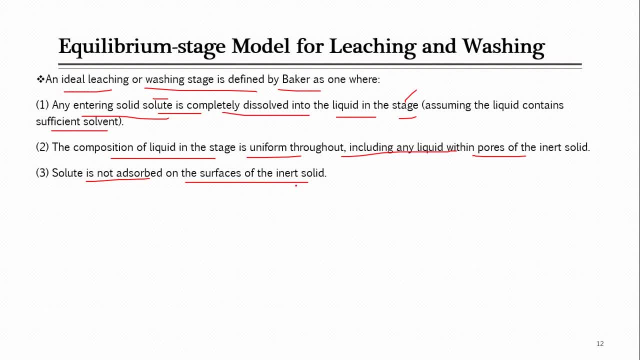 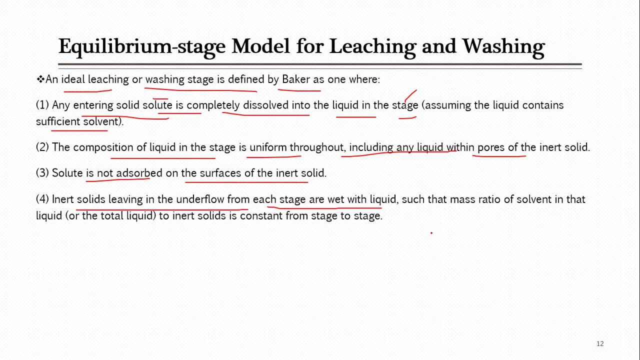 inside liquid, that is not, I mean, adsorbed on the surface of solids. Then there is next assumption: like inert solids leaving in the under flow from each stage are wet with the liquid, So inert solids leaving in the under flow, these inert solids which 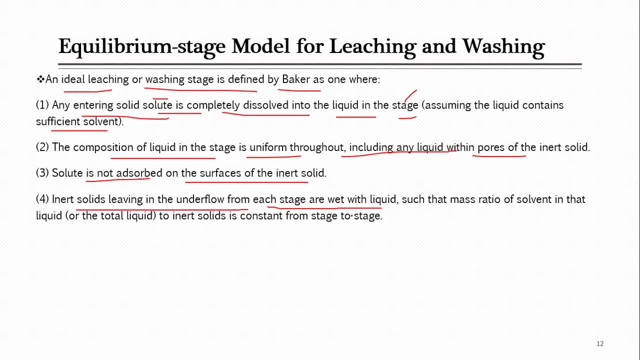 did not mean dissolved, So leaving in the under flow from each are wet with the liquid. I mean they are not dry, they always will contain some liquid, Such that mass. So the mass of the solid which is absorbed from the surface of the 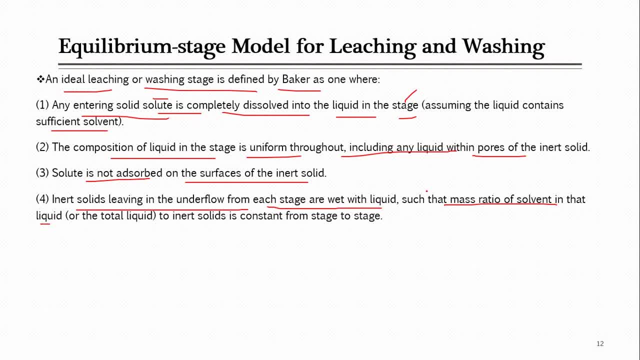 solid. So the mass ratio of the solvent in that liquid. I mean mass ratio of the solvent in that liquid or the total liquid, Suppose this liquid will contain more than one component. due to this he is saying like solvent in the liquid or the total liquid to the inert solid. 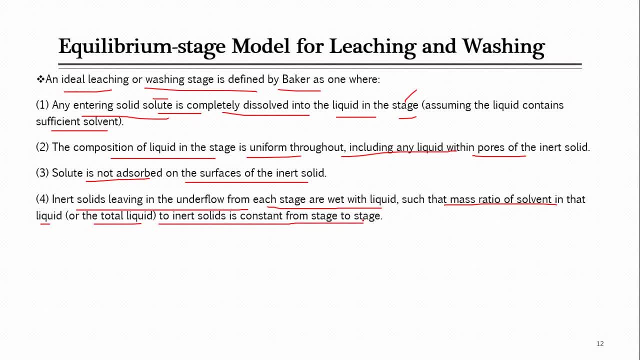 is constant from stage to stage. What does this means? It is mean, like, if you take the ratio of the- I mean mass- of this solvent to the- I mean solid, this remains constant throughout this. So it is obvious from here, if you remember, we said that inert solid as will remain constant. 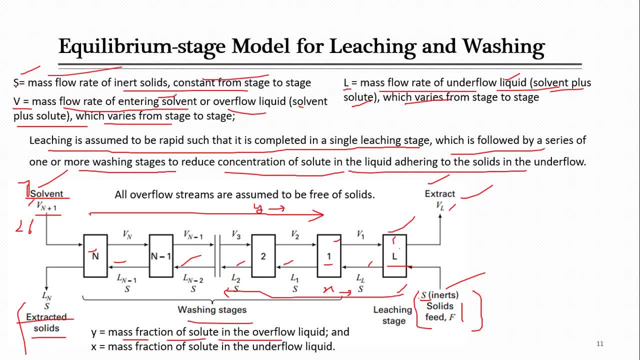 throughout. So when, as remains constant this when solid, specific amount of solids. suppose you consider that this is 1 kg of the solid, So that will also carry some specific amount of the liquid. For example, it carries 0.5 kg of the liquid, So that 0.5 kg divided. 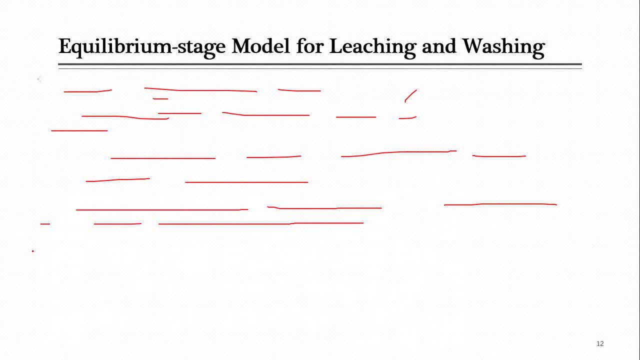 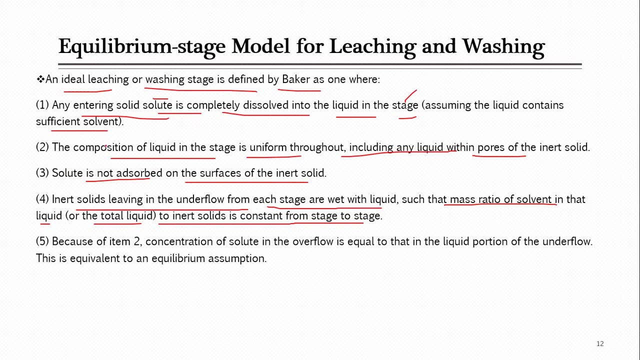 by this 1 kg. So it will be constant throughout the equipment, throughout all the stages, as he mentioned in this assumption. So, based on the assumption 2, which was what? that composition of the liquid in the stage is uniform in one stage, any stage which you just pick. So throughout that stage we consider. 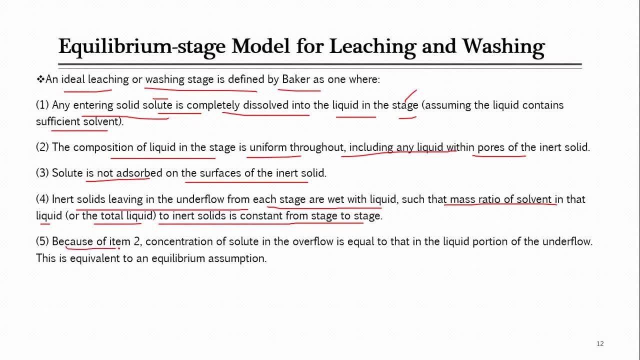 that composition of liquid is constant or uniform. So because of this point of uniformity, mean consideration, concentration of the solute in overflow is equal to that in the liquid portion of the underflow. This means, as I already told you, that when you consider complete 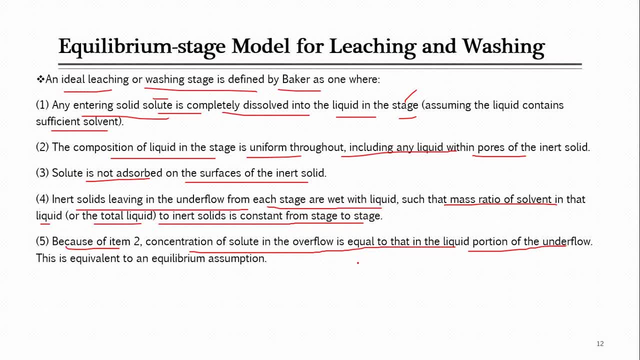 mix. Look at this source t e r continuous tank reactor. So in that reactor you consider anything which is leaving from this have the same composition as composition inside the reactor. So similar apply this here when any stream either it is leaving as the overflow. 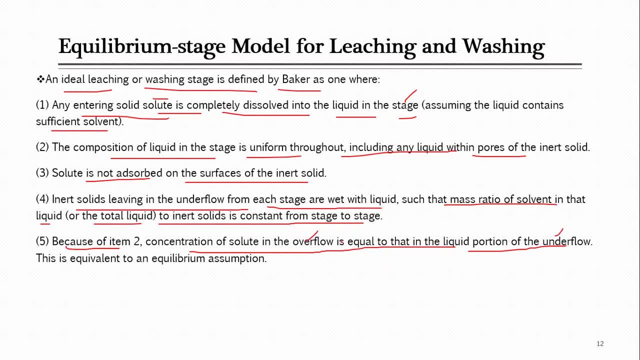 or underflow, it will have same composition. And when it will have same composition, meaning amount of the solute will be constant or will be equal- actually not constant, I should say It is. it will be equal, like either you take some sample from overflow from inside the 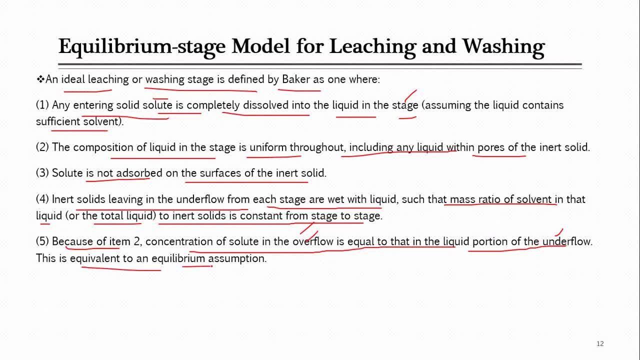 equipment or from under 5.. 3. nn. 3. under flow. So he says that this is actually equivalent to equilibrium assumption, which I already told you. Overflow contain no solid, as initially it was said that the inert solids are not, do not become the part of the liquid, So they do not leave as a overflow, they will. 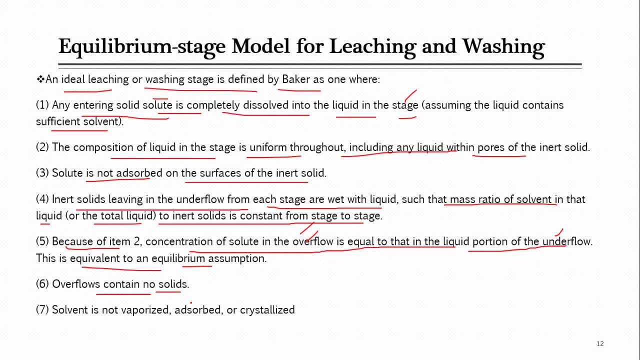 be only leaving as a wet solid and from the bottom of the equipment. Solvent is not vaporized. adsorbed or crystallized means solvent which entered from the first stage. I mean, I should say not first, it is n plus 1 stage, So that remains constant. 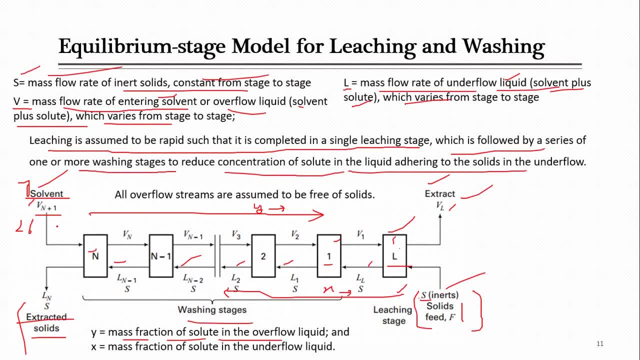 throughout the equipment. the solvent which entered from here is actually he, as he said mean. this enters, suppose, 1 kg, So it will leaving at the end somehow, I mean at the this stage, if last stage we just consider 1 kg will be distributed between this and the final. 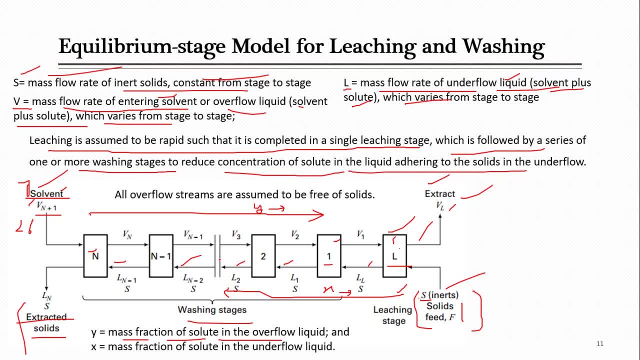 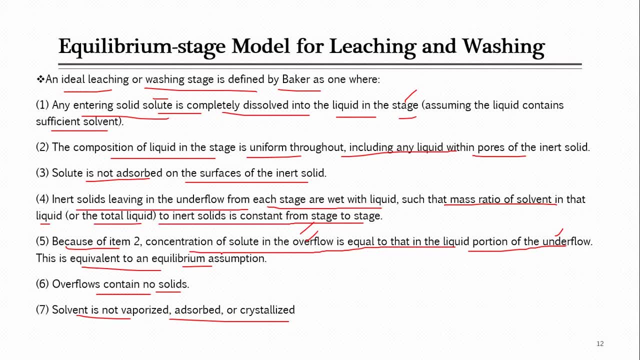 which will become part of the wet, But it is not like evaporated, it is not crystallized, it is not reacted throughout the whole system. So these are All assumption which are considered for this equilibrium state model for leaching and washing After this, if we- because we are short of the time, this is the last lecture, So I have. 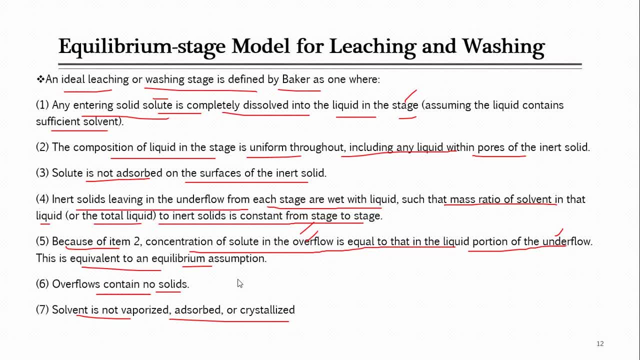 to finish, stop it here. but only one topic of related to this leaching was like: suppose if we have another lecture we can easily do that, that is, its use of all these assumption for the mass transfer and then, and this mean to solve numerical problem. but already you. 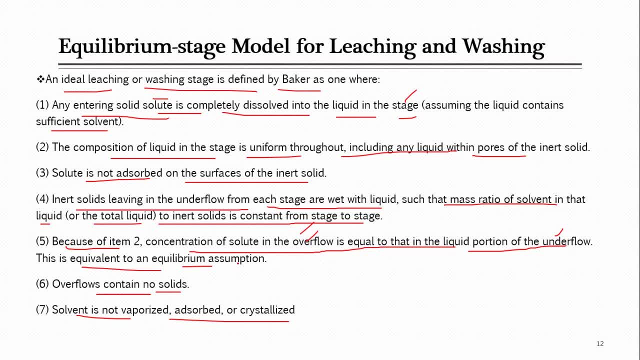 have done a lot. So just go through all those stuff means try to solve those problem. leave its problem just. you should know the theory, you should be aware about its basics at least. and all this stuff if we have discussed, especially this, I mean countercurrent equilibrium washing. 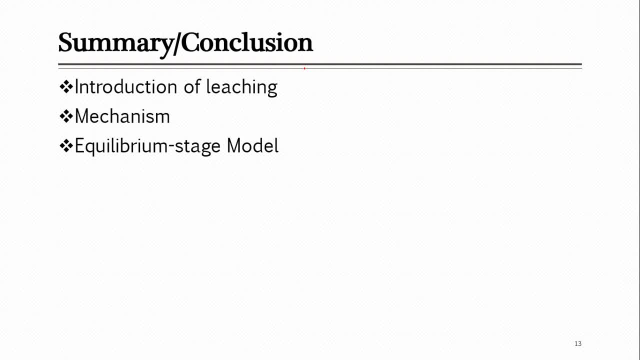 model. So thank you so much. I will just summaries all the stuff which we started like. leaching is also called liquid solid extraction, in which you bring in contact, once solid, with the liquid and the purpose is to extract some part of the solids towards liquid. So we 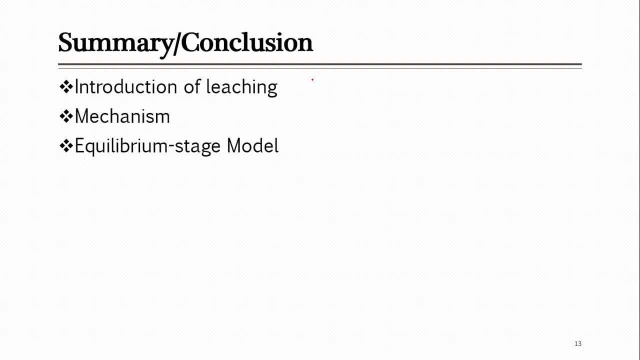 can just get them separated. and then we we have seen the mechanism. how does it take place? they come in contact, they mix with each other and later you get them separated and the top layer is the overflow or extract mean, which is the liquid containing or the solvent containing some. 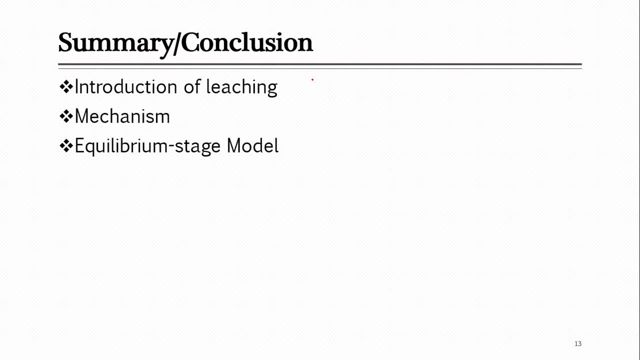 solute and the from bottom, usually solids, are living as a wet mean wet solids. so then we have seen at the end the equilibrium stage model that's counter current model most widely used. for these i mean techniques, and that shows that usually you will have one leaching stage, but there are 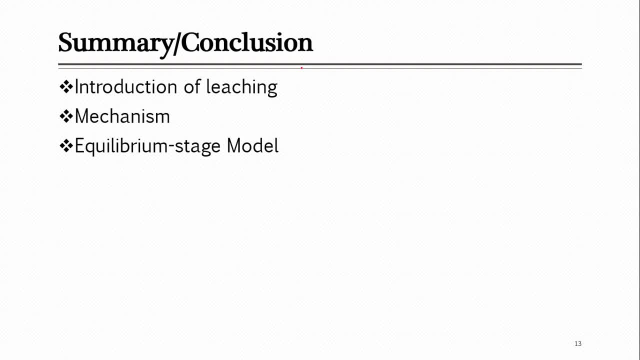 number of washing stages and washing in washing stages. actually you are decreasing the amount of solute which is being carried with the wet solid- and here remember that solid didn't absorb anything of those solute- and actually this solute is being carried out with the liquid which is part of wet. 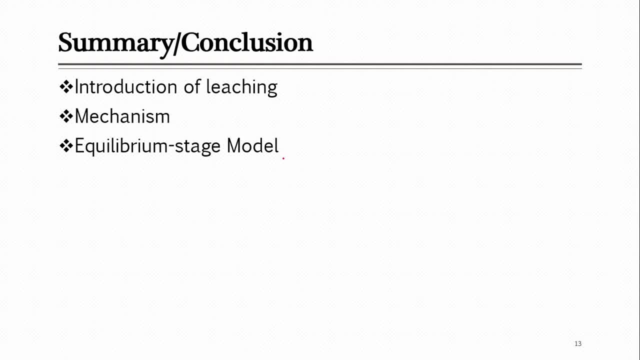 solid. thank you so much, and all office you.